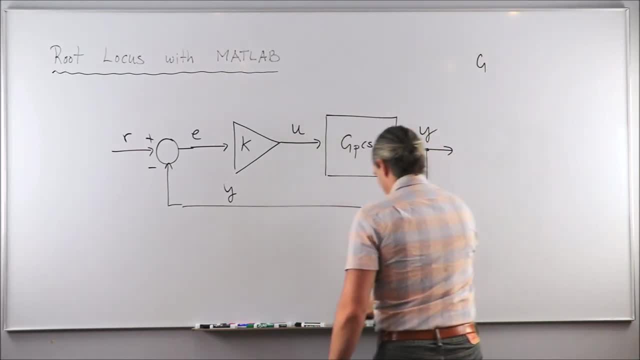 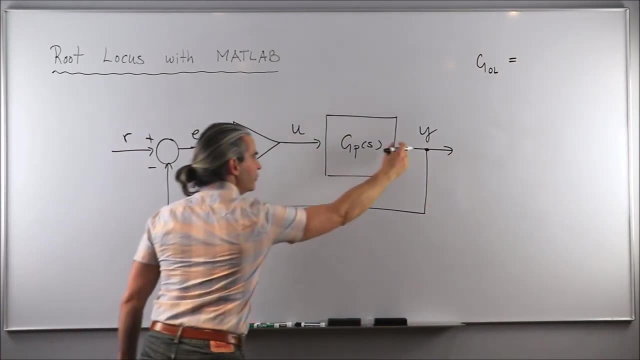 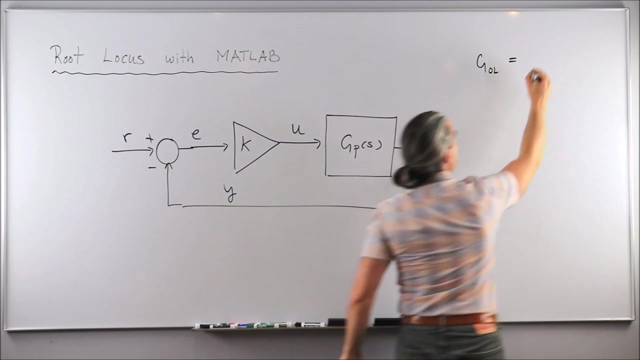 open loop transfer function: g open loop, which in this case we're going to use: the g loop transfer function: g open loop. So in this case, if you neglect the feedback loop here, all you have is k, the proportional control gain that multiplies our plant transfer. 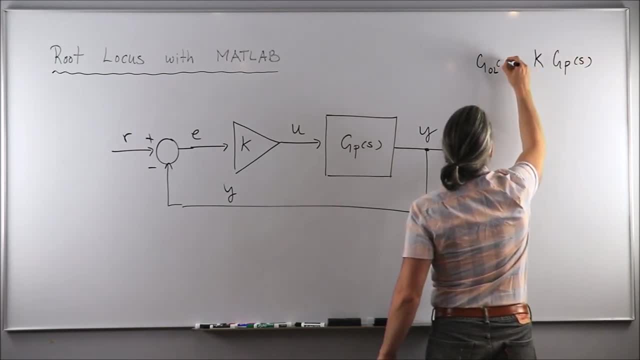 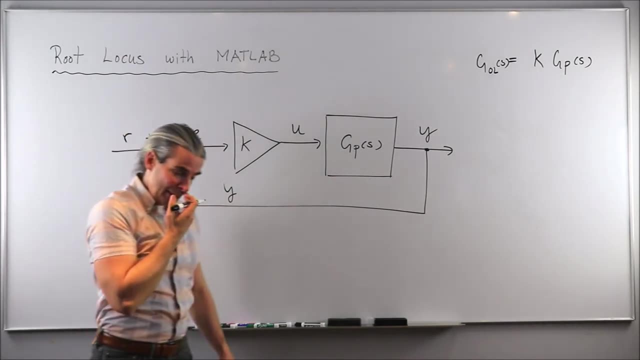 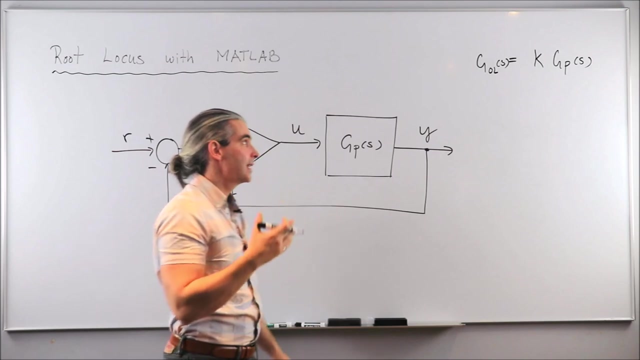 function g of p. okay, Like that. But then we said, okay, the root locus being a visual mapping of all the closed-loop poles, we're going to use the g loop transfer function g of p, okay? So if we look at the holes in the close-loop poles, it means that we needed 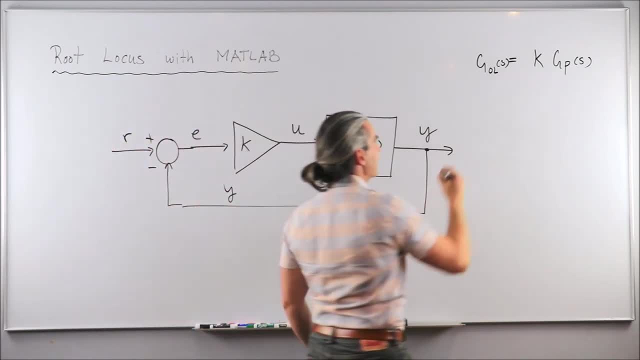 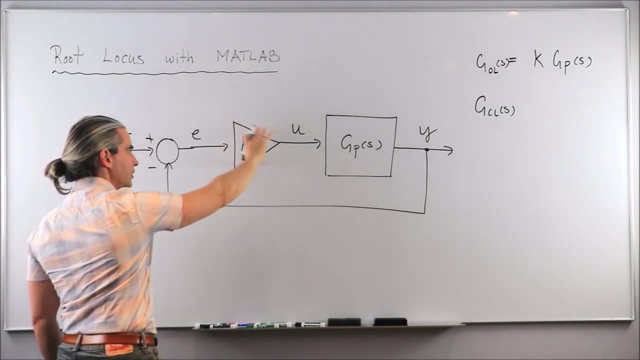 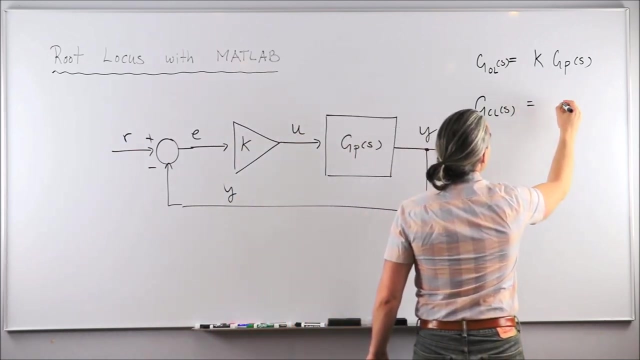 to obtain the closed-loop transfer function. Fine, our closed-loop transfer function using this feedback configuration, where you have a control gain in series with the plant and then again the feedback move closing. everything was simply g open loop over 1. 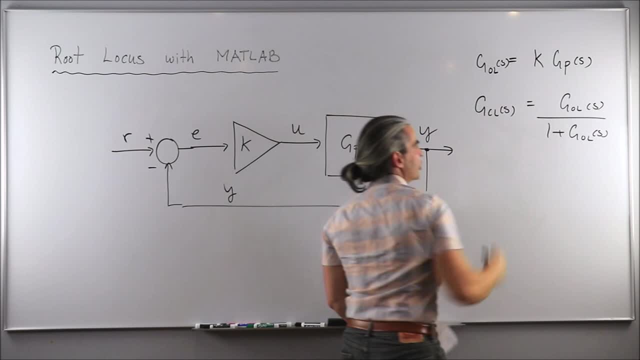 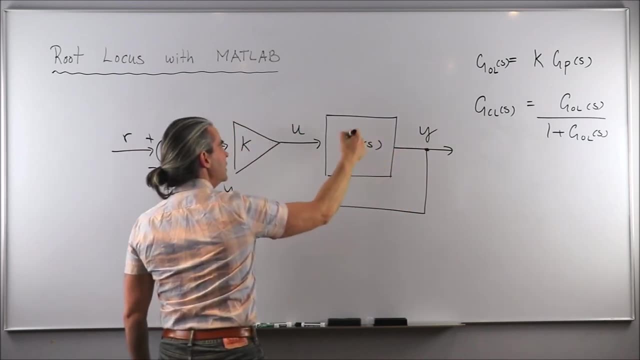 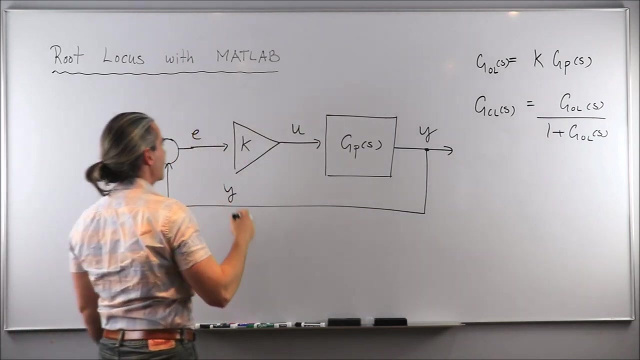 plus g, open loop, And if you're not sure how to get that, you just, you know, write all the signals. so y is equal to g of p times u, u being k times error, error being r minus y, and then you solve for y on one side and then you obtain the transfer function. 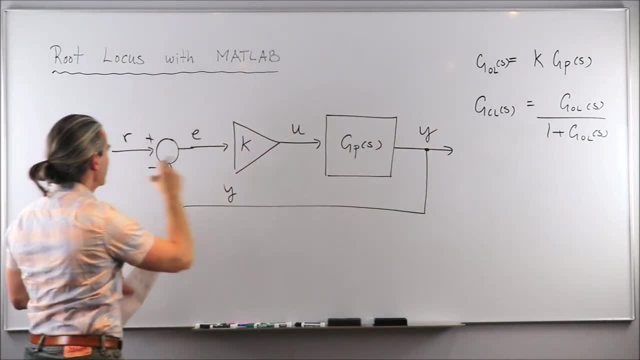 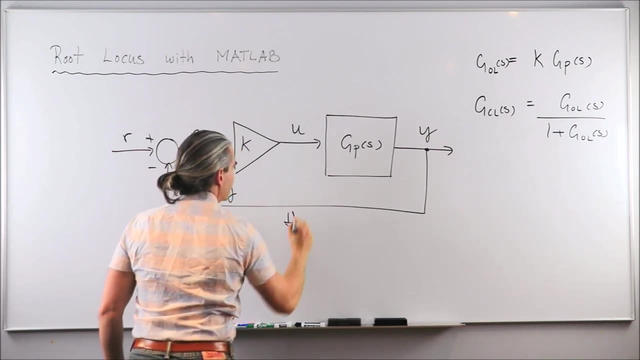 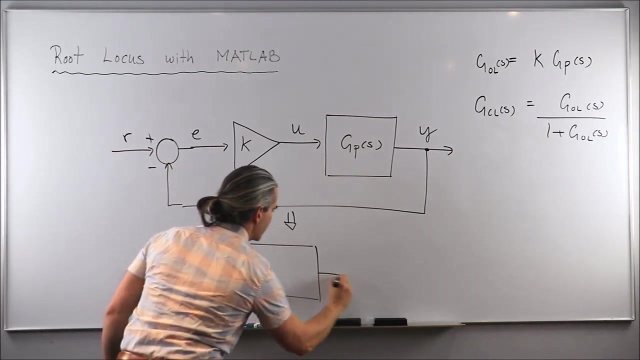 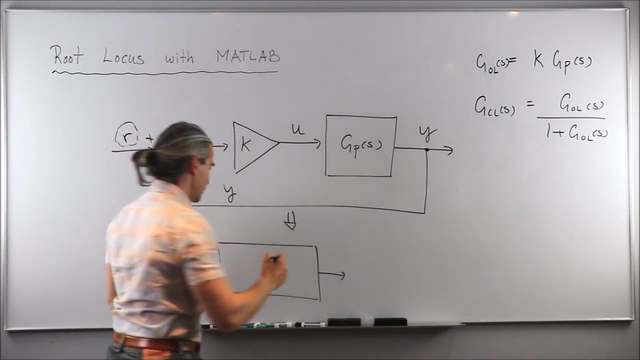 between y and r as being global output and global input of everything. so that was a closing transfer function, meaning that this system can now be represented by a single transfer function that does the mapping between this, what i call global input, r, and widening the global output. okay, 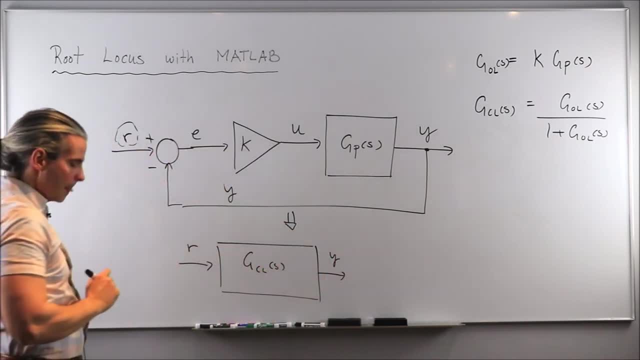 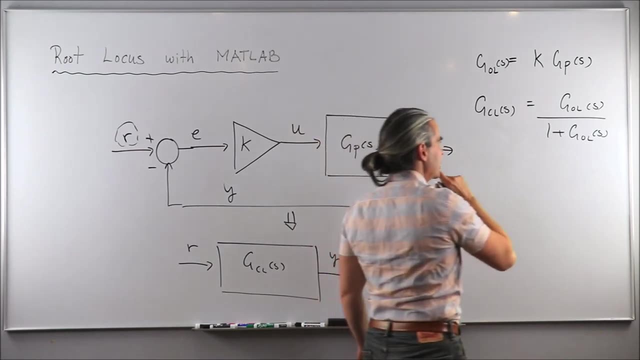 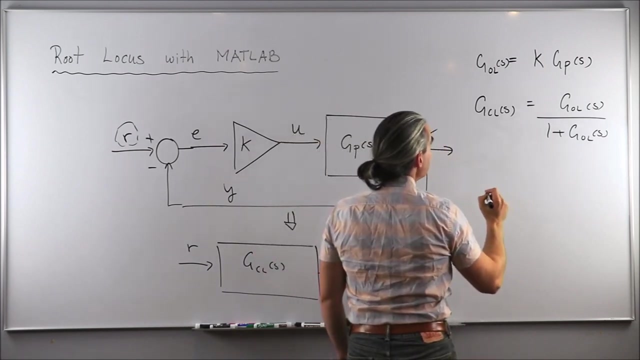 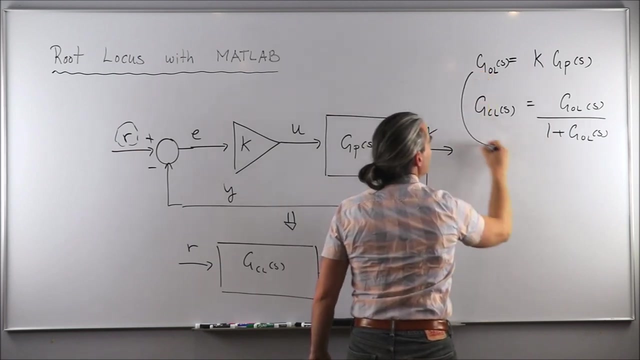 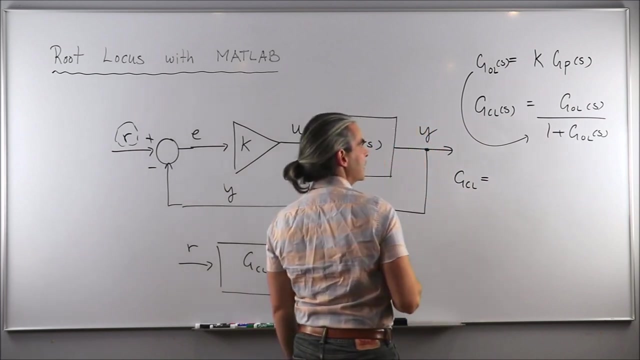 g closed loop transfer function like that- all right, but then we needed to get the poles of that transfer function, so the first thing we did was to substitute g open loop inside of it, so g closed loop. i'm going to drop the function of s for the follow-up development, just to ease up. 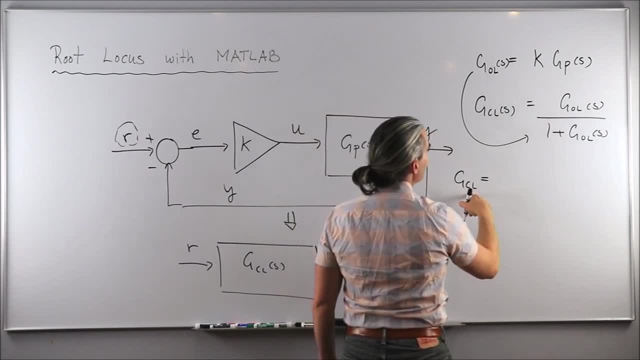 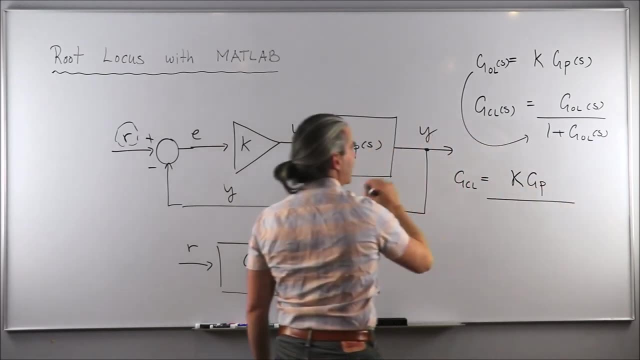 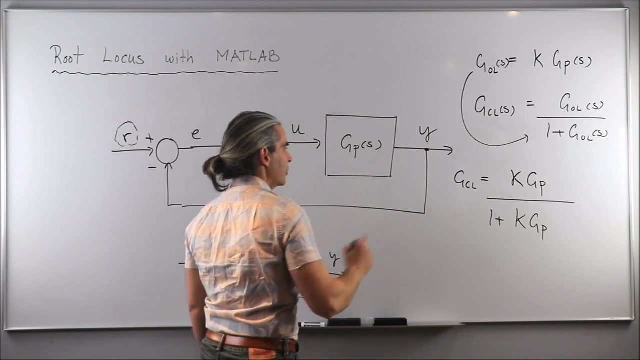 the nomenclature of it. so g closed loop, g open loop, meaning that this is k times the transfer function of our plant over one plus g open loop, being k plus g of p. okay, good, now i'm in a position to obtain my characteristic equation, which is nothing more. 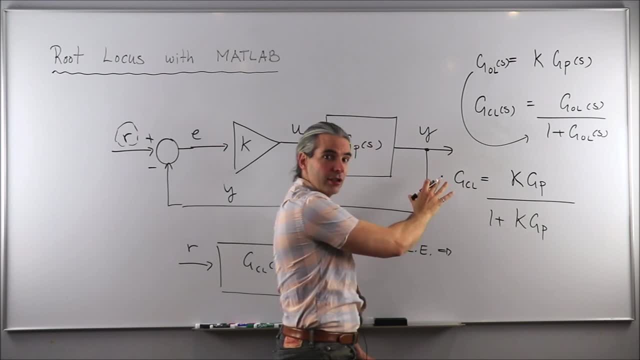 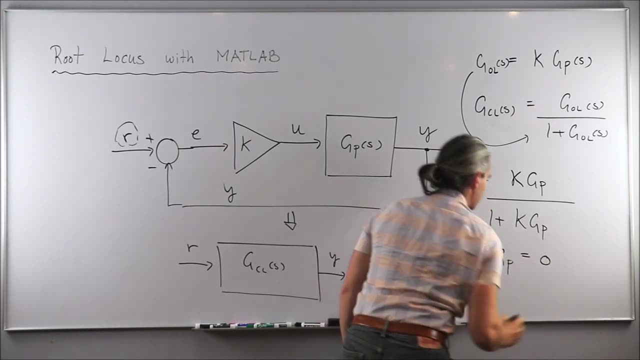 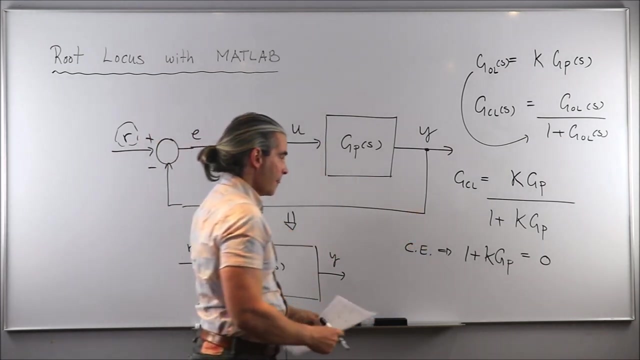 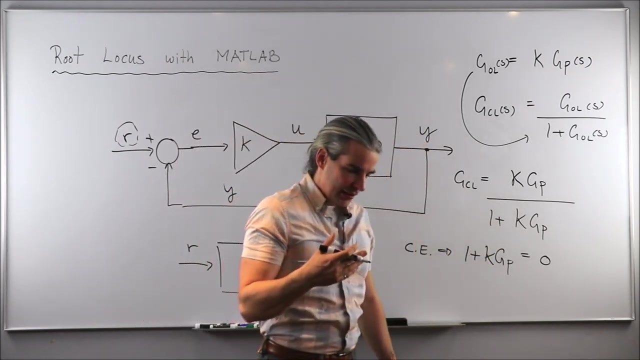 than just the denominator of my closing transfer function set to be equal to zero. that's one plus k times gp, equal to zero. all right, now, there was also the discussion that whenever k was being set to be equal to zero, what we get is actually the poles of the open transfer function. 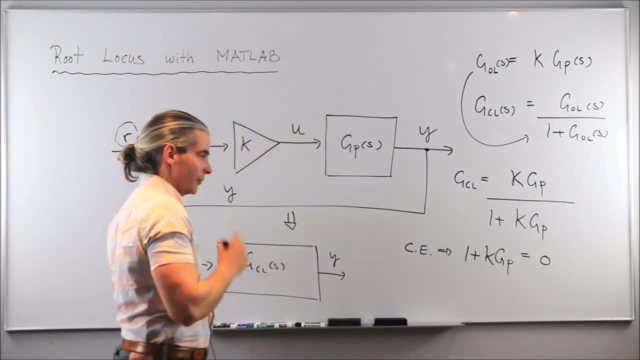 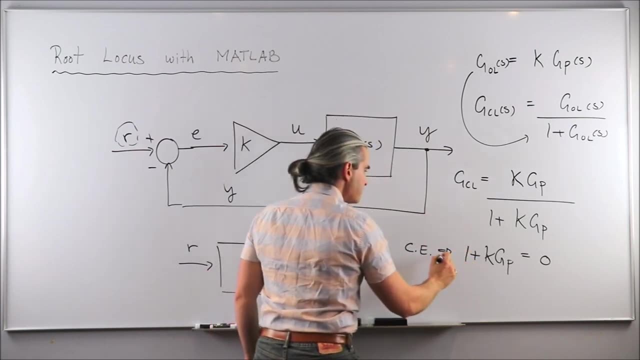 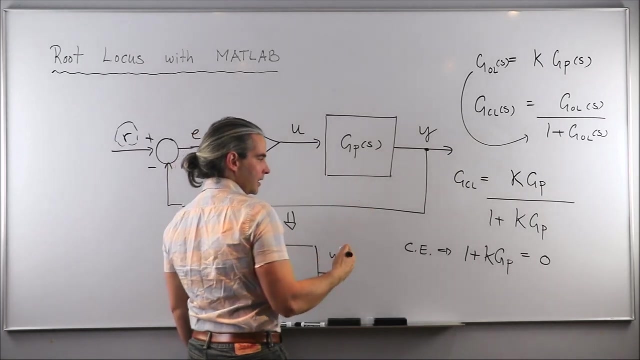 as opposed to the poles of the closed transfer function, and i'm going to come back to that notion in a second, but just for the time being, looking at that, it means that all we need in order to map the poles in a complex plane is to solve that equation for its roots. 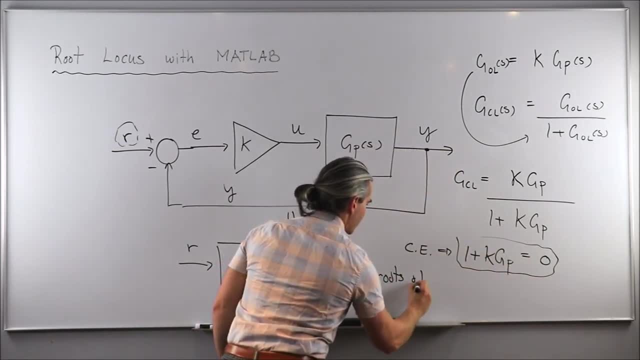 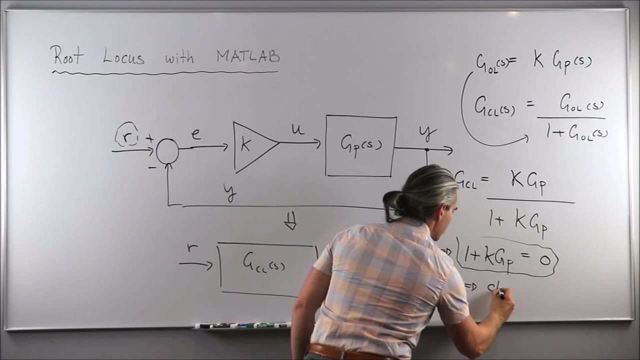 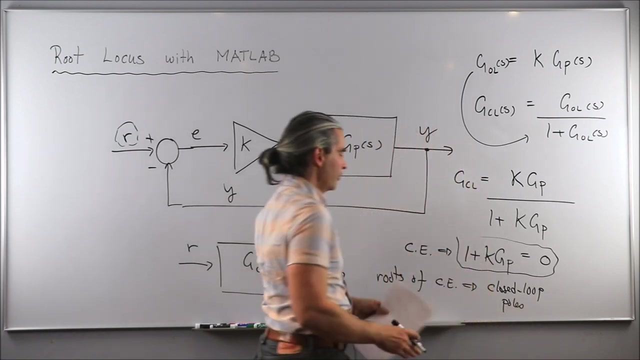 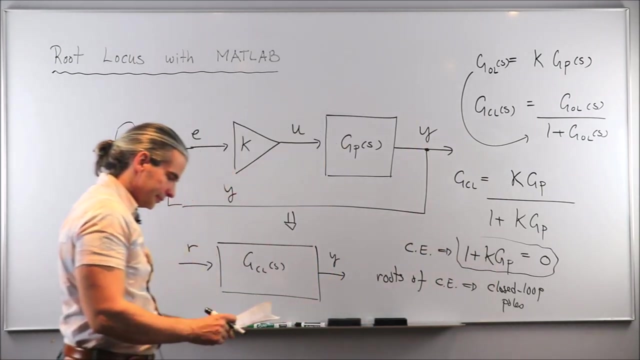 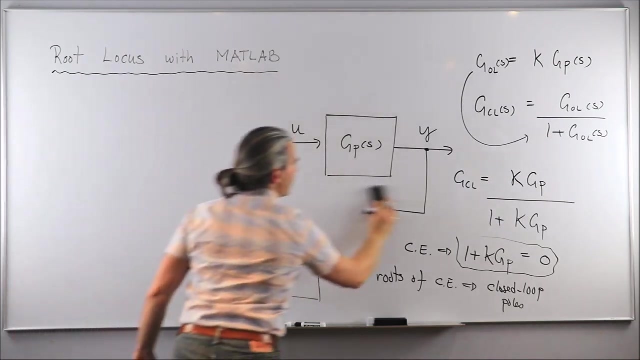 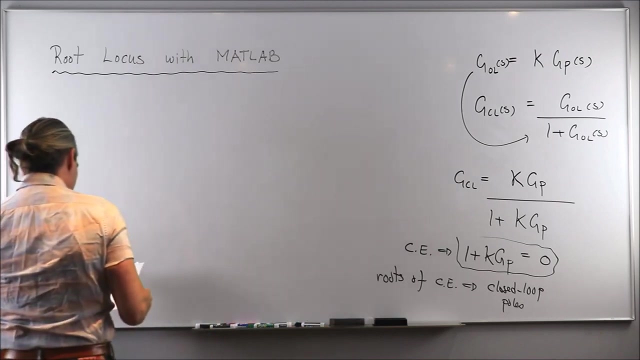 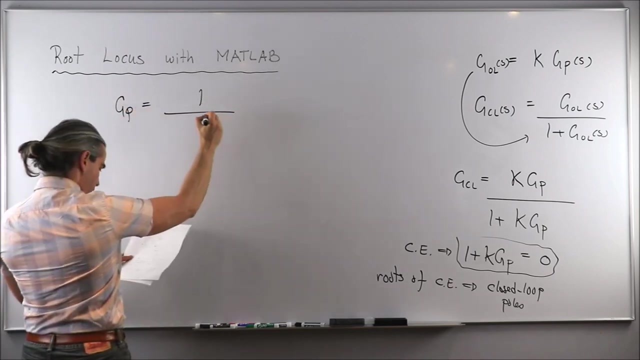 okay, so the roots of our characteristic equation actually correspond to the closed loop poles for various k values, from zero all the way to infinity. excellent, and then we had looked at a particular example. just put that in context. our first example we had solved. the root, locus four, was gp equal to one over s of s plus one. 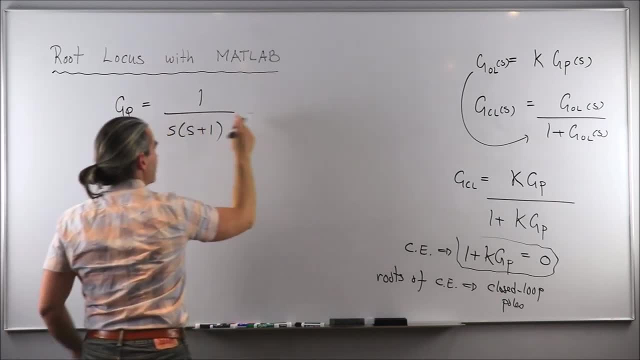 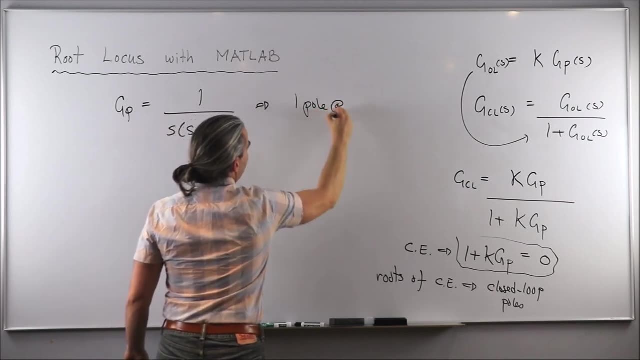 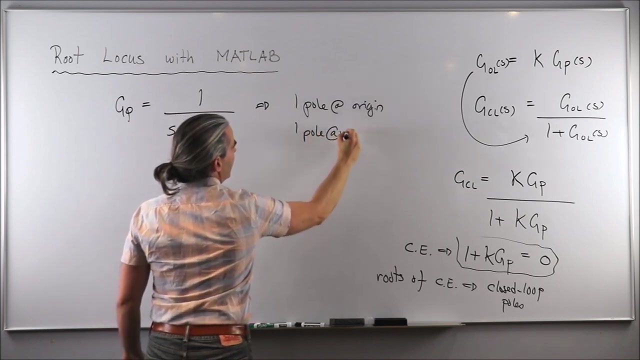 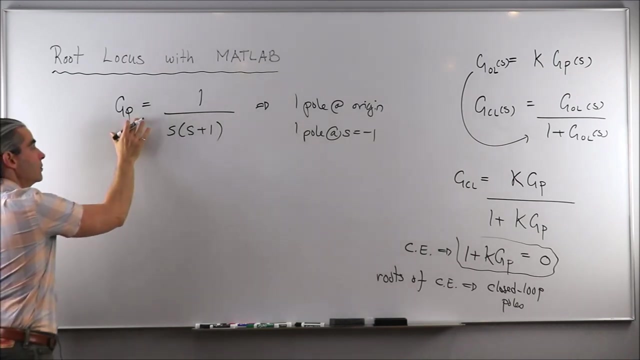 meaning that just the plant itself, with no control action, no feedback loop applied to it, had one pole at the origin, the complex plane, and then one pole s equal minus one. but that's for the open loop or the just plant on its own. nothing else applied to it, so that's a good. 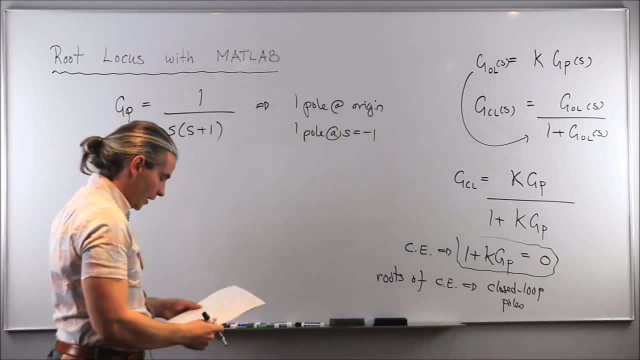 piece of it here in this example. but now that we know that we have one pole and we already have a second one, we can apply that and apply that to one of these things here with the via for loop zero to zero, and we would have one pole, and we would have a negative pole, and then one pole and we would have 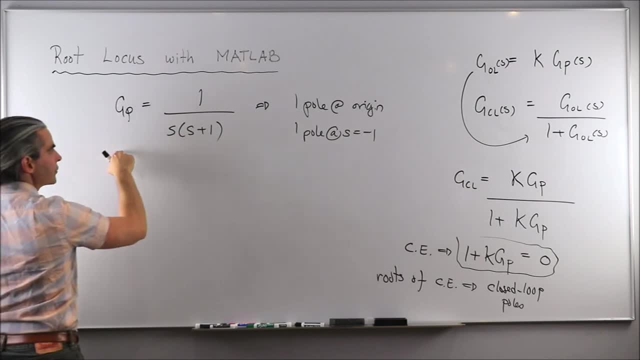 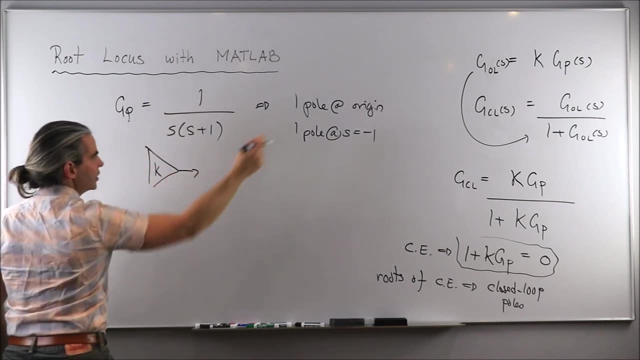 a negative pole and we have the same situation. but this is actually the opposite of the original plan. but for this then we had obtained the closed transfer function. by multiplying this plant with control action k, as i just did previously, because k multiplies gp, i produce a new output. we feed this back. 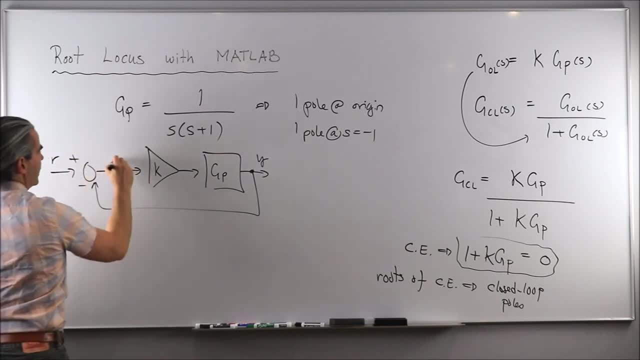 compare that to the reference signal. that creates an error and multiplied with k gives us a control input signal u. so we have taken that, obtained the closed transfer function and looked at the characteristic equation just like what we did here and we had obtained for that specific example a. 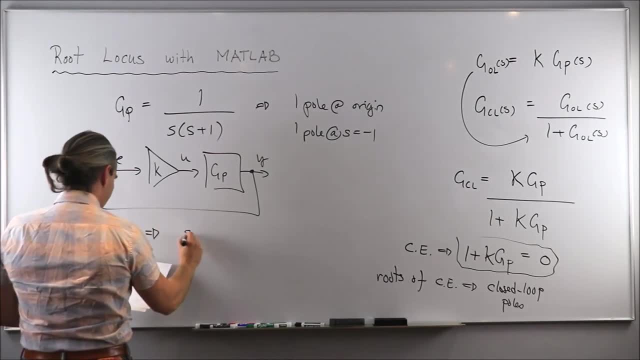 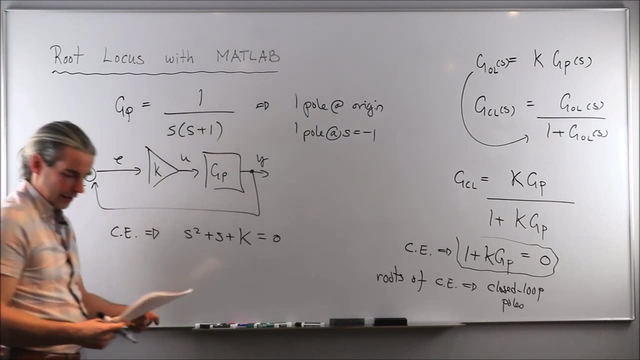 characteristic equation that was s square plus s plus k, equal to zero, if you remember the example we did together, i right? so that gives us the poles of the closed loop transfer function, because this again is characteristic equation of the closed loop obtained as being g open loop over one plus. 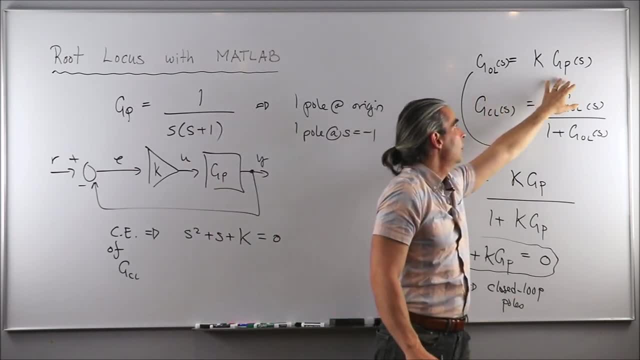 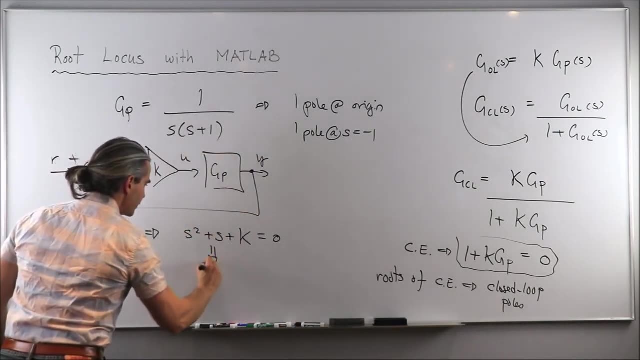 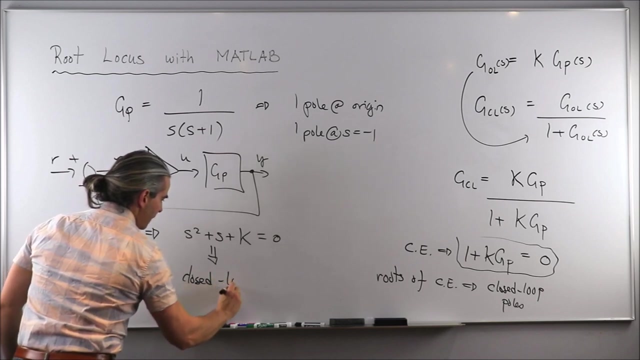 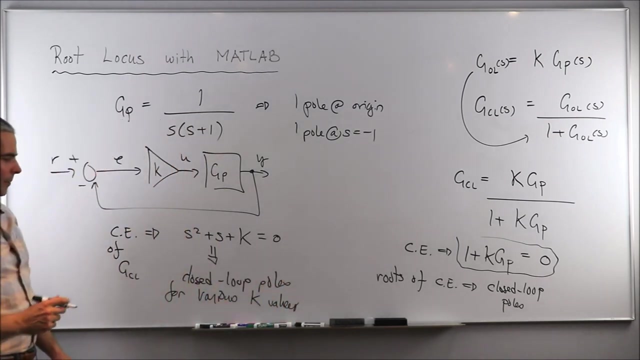 g open loop, and g open loop being our gain, multiplying the plant transfer function, essentially solving for the roots of that. give us same thing: the closed loop poles for various k values. but how does that relate to the open loop position when k is equal to zero? well look, 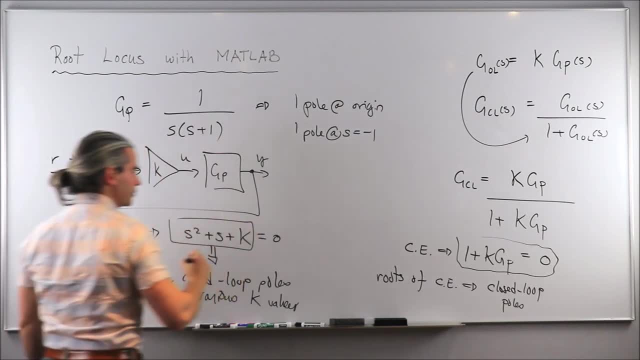 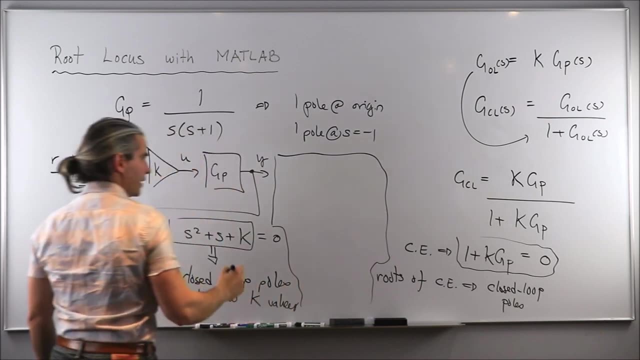 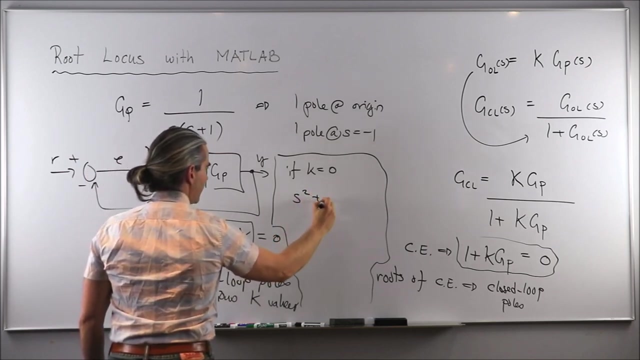 if you take that and you set k equal to zero, you get the two poles for the closed loop position and i'm going to do this work in this little box here, running out of space. i'm gonna say f, k equal to 0. on that equation you get s square. 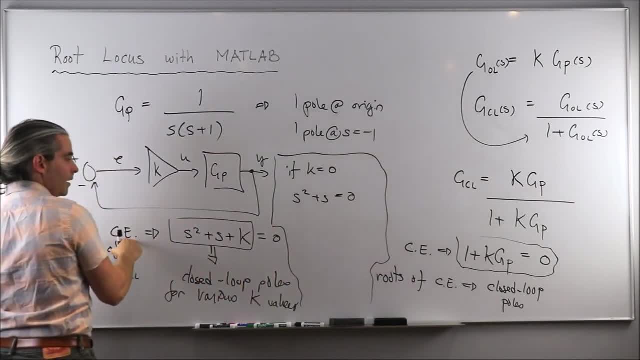 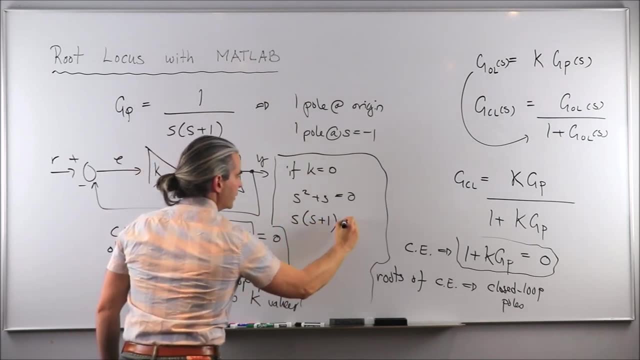 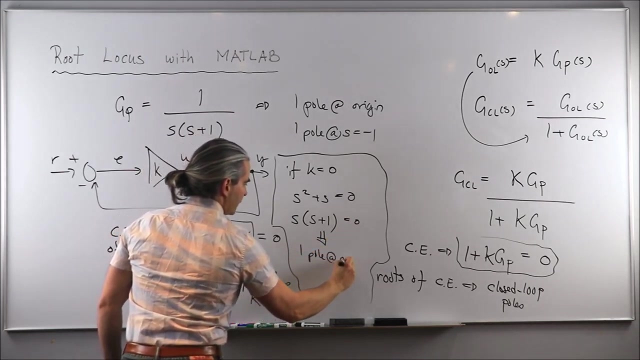 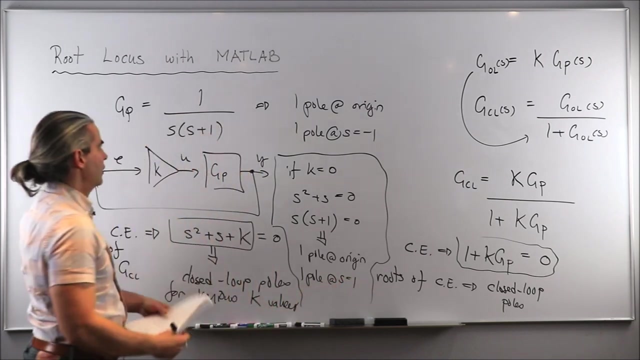 plus s equals zero. for the characteristic equation evaluated specifically at this point here, or in other words, s times s plus one equals zero, and obviously that gives us two poles at the origin of the complex plane and another pole at s equal minus one. and look at what we. 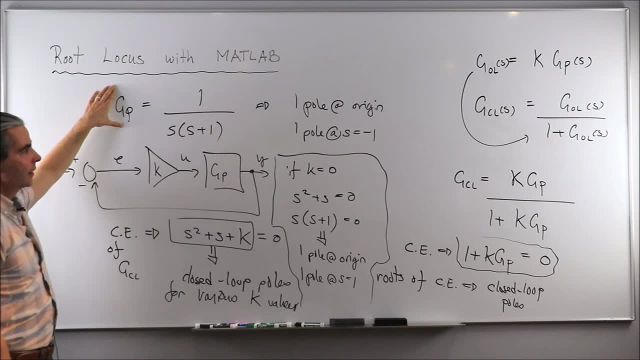 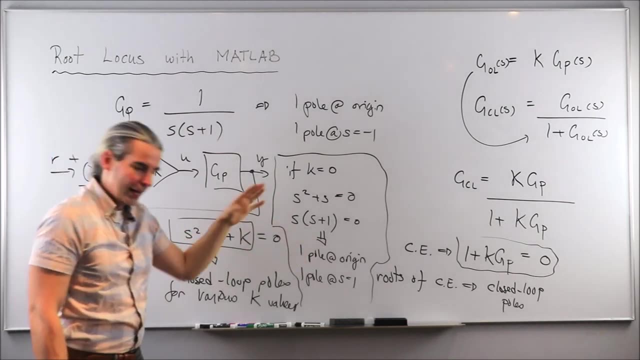 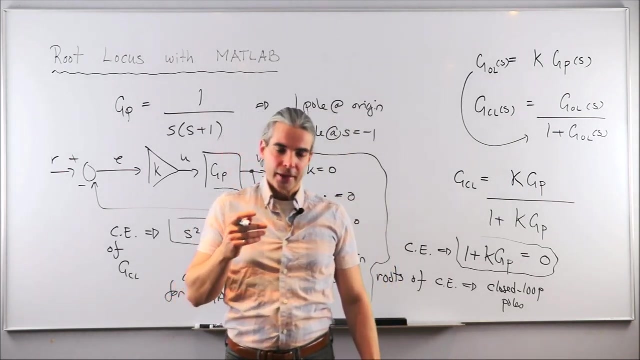 had to begin with with just the plant on its own, in an open loop fashion: one pole at the origin, one pole at s minus one, exactly the same thing, and that's why i said back then that the root locus is a visual representation of the poles at, while starting from k equals zero. those correspond to. 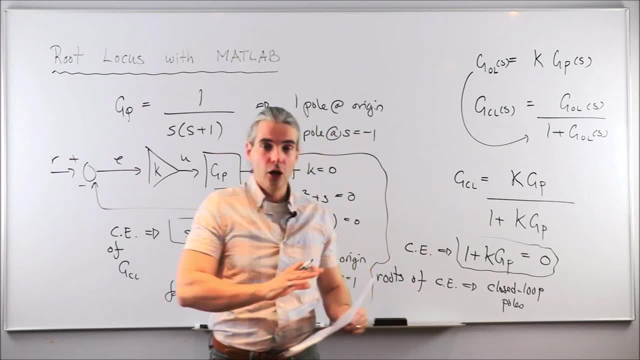 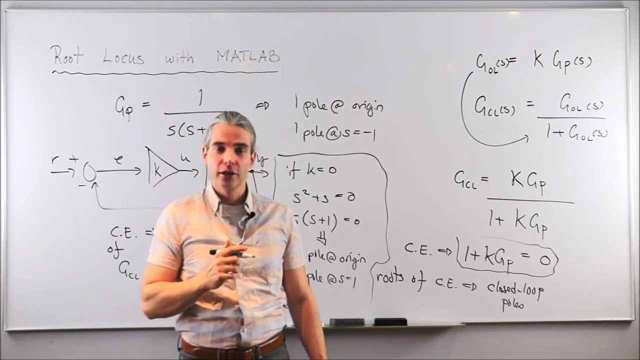 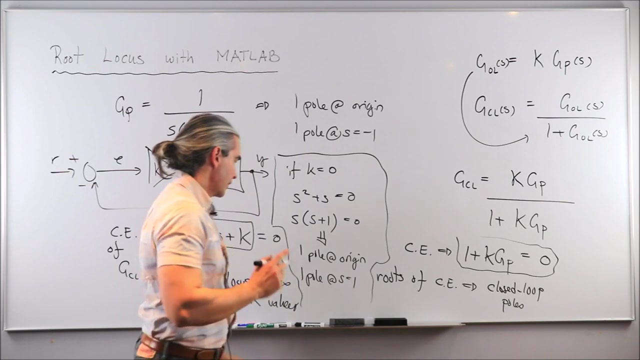 the poles at of the open loop transfer function all the way to infinity. so as soon as the k value for the open loop gain that multiplies the plant transfer function is increased beyond zero, you don't get the open poles anymore, you get the closed poles. all right. so an obvious solution. 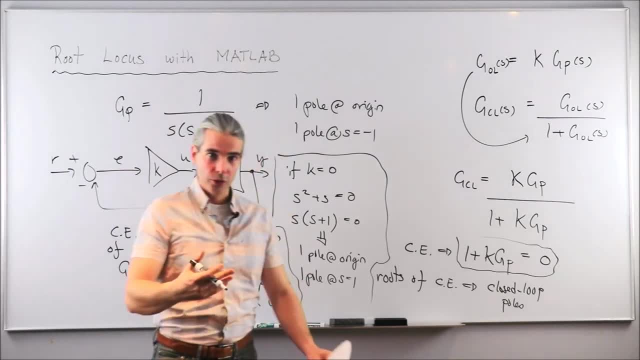 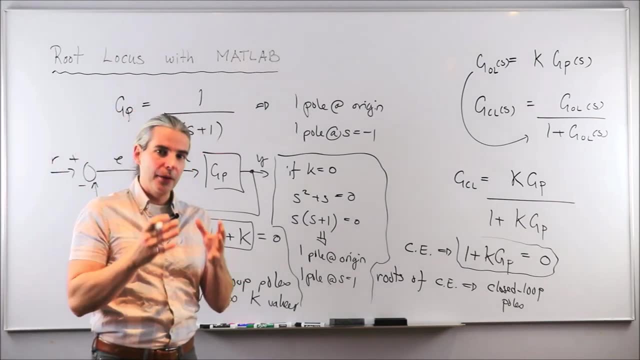 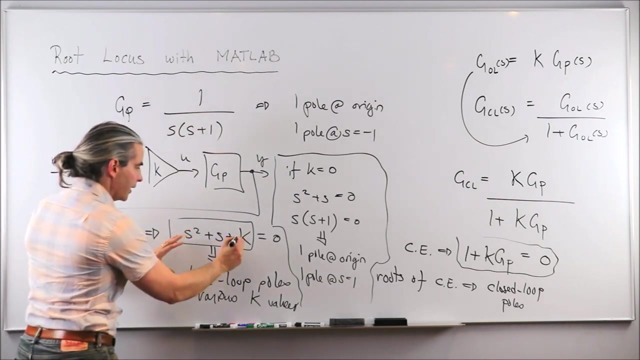 is to use matlab to obtain a root. locus is simply to calculate or to first obtain the characteristic equation of the closed loop transfer function and then, varying the gain k for that characteristic equation and for each iteration for k value, obtain the new roots of that equation and those 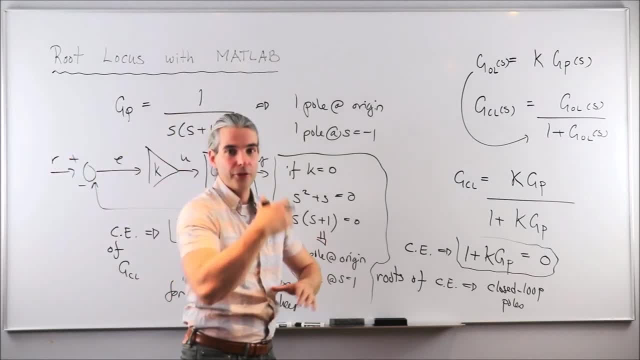 roots will correspond to the closed loop transfer function. and then varying the gain k for that characteristic equation and then varying the gain k for that characteristic equation, the holes when every k set to be larger than zero at k is equal to zero, you get the starting point. 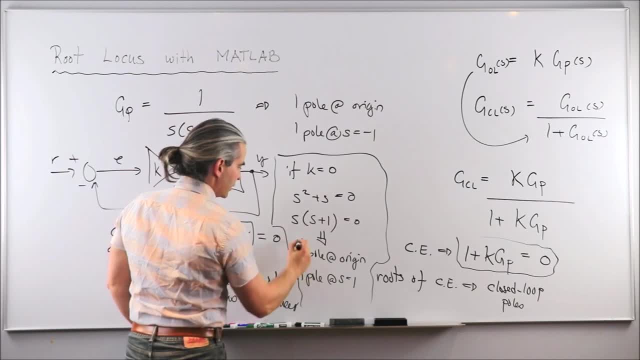 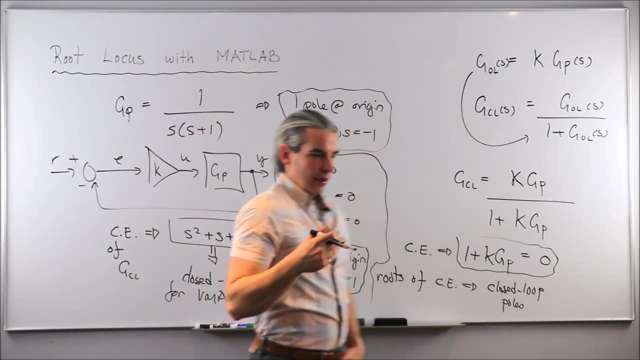 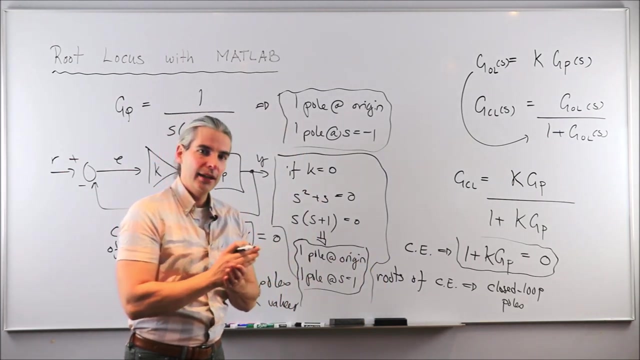 of the root locus, which is what you had originally, with just the plant. same thing, okay, so let's go to the computer, let's use matlab and let's brute force the calculation of the root locus by calculating the roots of the characteristic equation for this specific example, for each variant of the root locus. 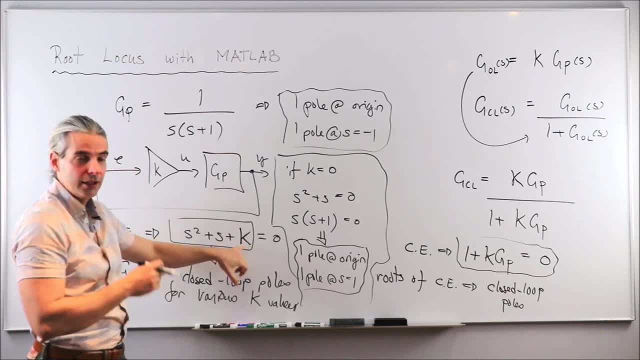 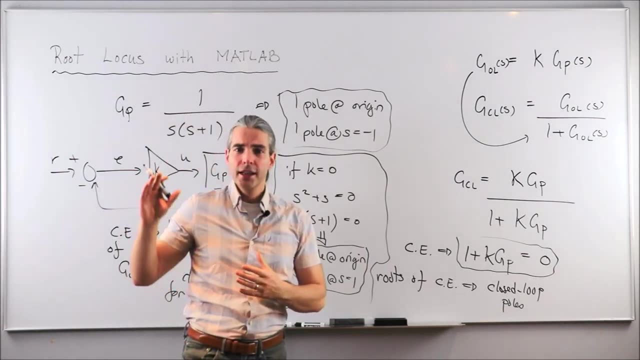 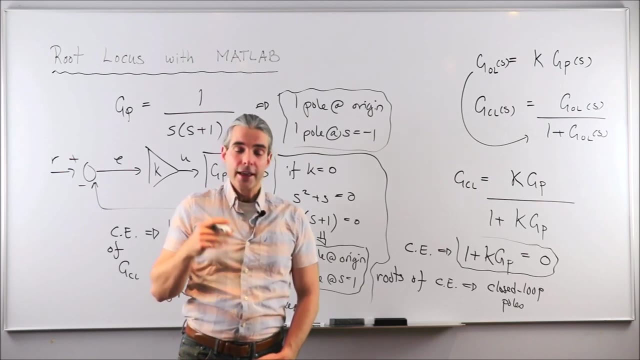 value of k, considered from zero to some large values, and let's map or let's plot those roots inside the root locus and let's compare that to the hand-written solution we came up with in the previous lecture. That's the first thing we're gonna do. 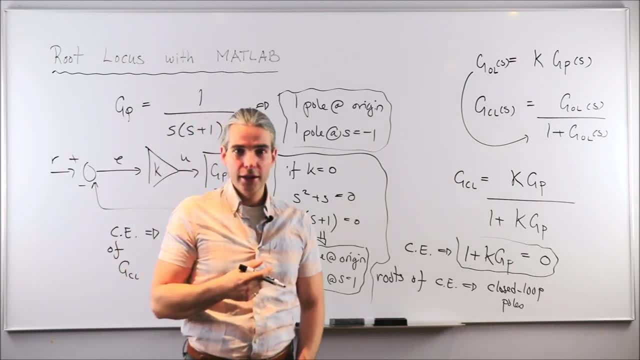 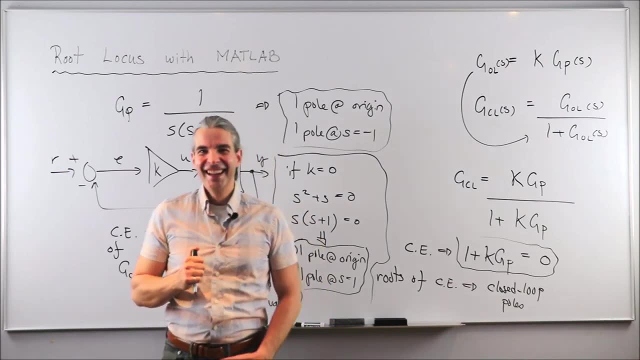 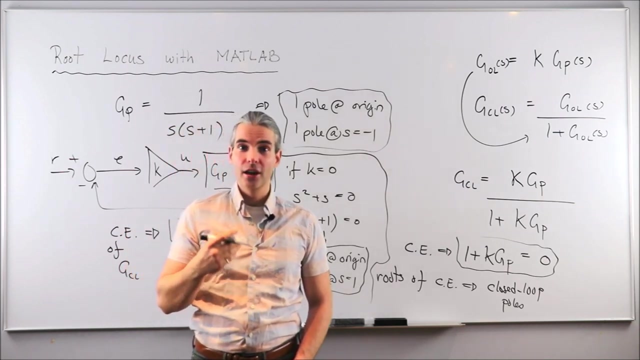 Then we'll ask ourself: is there a better way to do that, using MATLAB? And the answer is obviously yes, Otherwise I wouldn't be asking you that question. okay, And that solution simply uses the MATLAB built-in function known as rlocus. 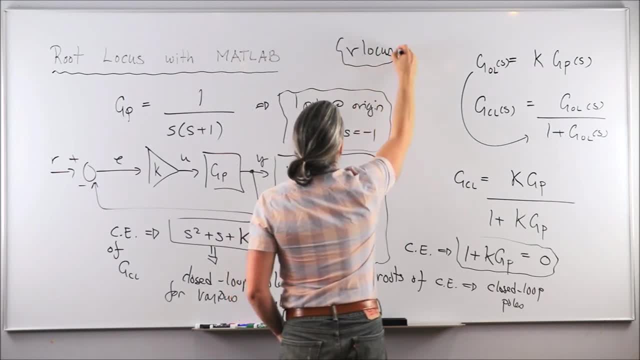 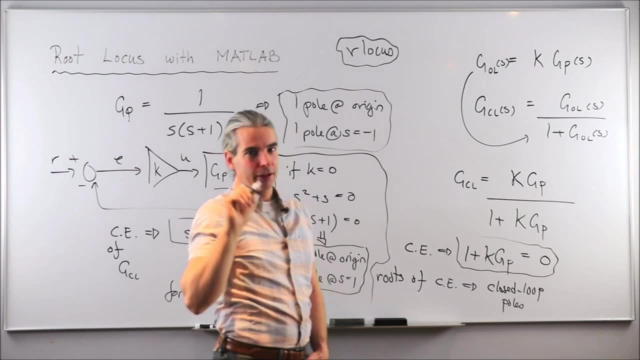 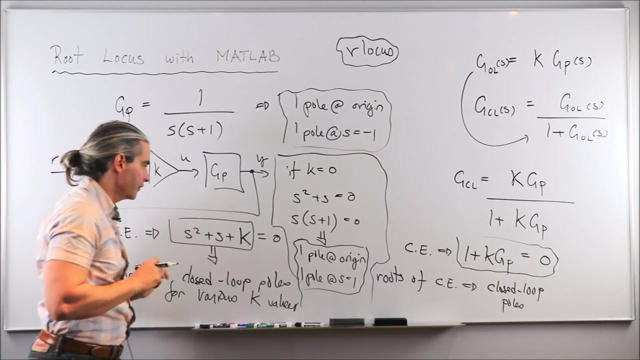 So rlocus, being a MATLAB command that you can use, will draw the root locus automatically for you. But first thing, first, let's brute force the calculation by obtaining the characteristic equation solving for its roots at each value of k that we're gonna construct. 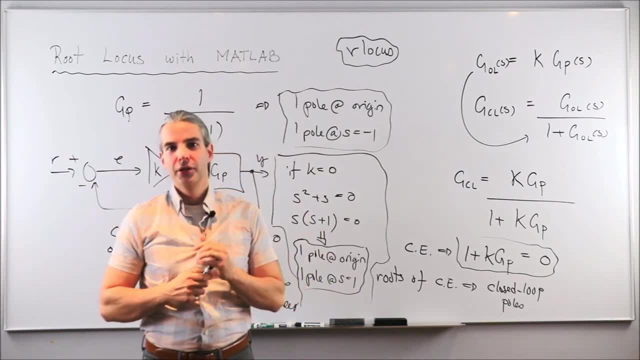 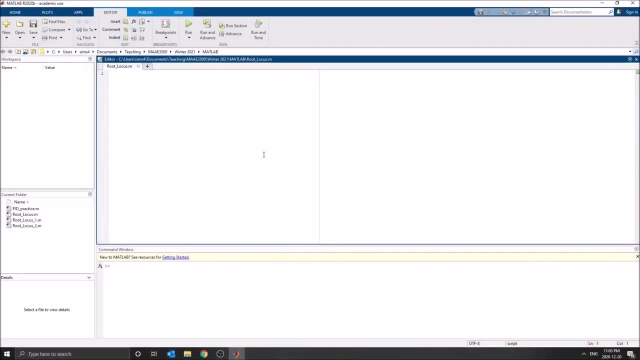 That's it All right. so let's go to the computer and let's do that together. Here we are in MATLAB and, as mentioned on the whiteboard discussion, we're gonna use that software to create the root locus for us instead of doing it manually. 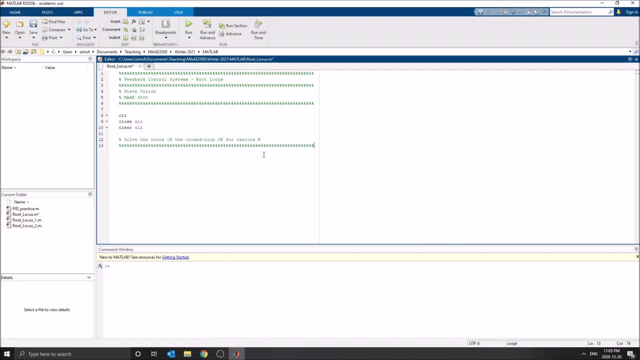 following all the nine rules we saw in the previous lecture. So first things first. I always like to start any programs I write in MATLAB with the CLC close all and clear all commands, which respectively clears the command window, So it will clear all the commands from any type commands. 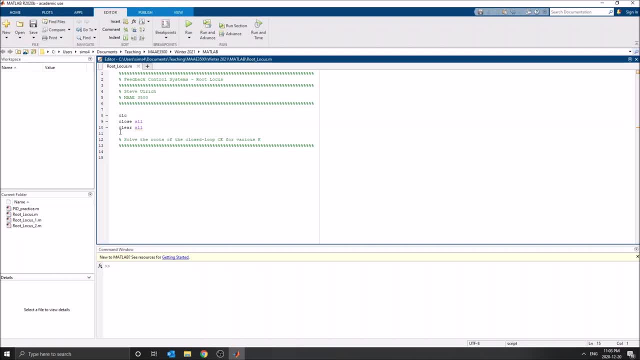 will close any open figures and will clear any variables we have in the workspace. So it's just a neat way to start fresh, essentially. So, as mentioned in the whiteboard discussion, the first method we'll look at to create a root locus. 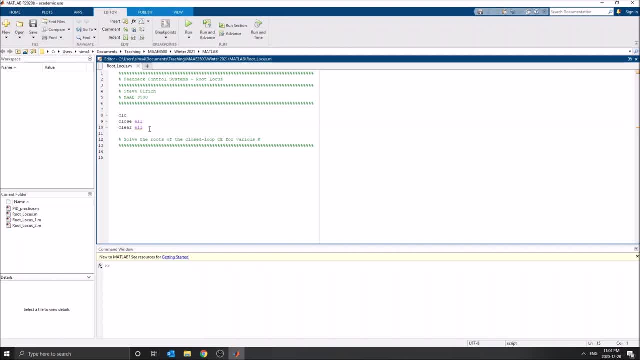 using MATLAB is the brute force approach, which simply consists in solving the roots of the closed loop characteristic equation at various gain values. first create a new figure and then we're gonna say: hold on, so that we're gonna give us the ability to plot multiple poles for each gain value. 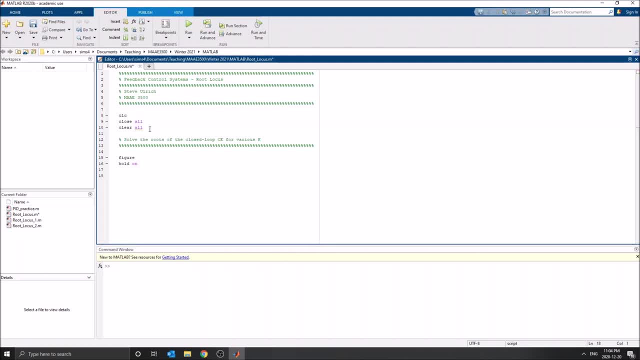 at each iteration on the same figure. So let's start the for loop within which we're gonna do the calculation of the root of that characteristic equation. So K, beginning at K, equals zero, or in other words, at the open loop, pole locations. 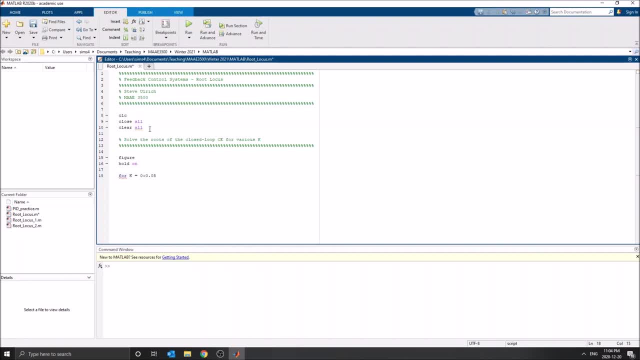 then we'll start increasing our gain value, say with 0.05, all the way to 0.6 is gonna be sufficient to see the general behavior of the root locus for the first example that we've looked at. Okay, and then I'm gonna end my for loop right away. 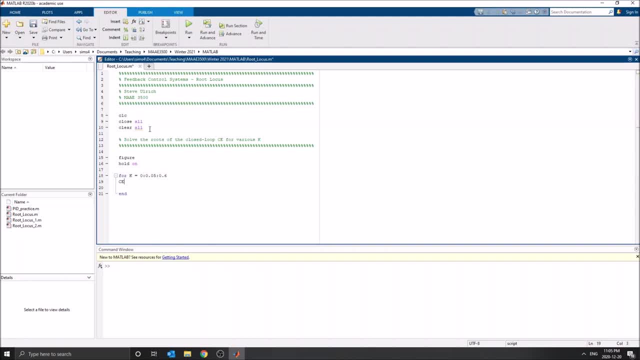 so that I don't forget about it. So the first thing we wanna do is to define the coefficients of the polynomial. that corresponds to our characteristic equation of the closed loop transfer function. In our case it was S square plus S plus K. Do you remember the example? 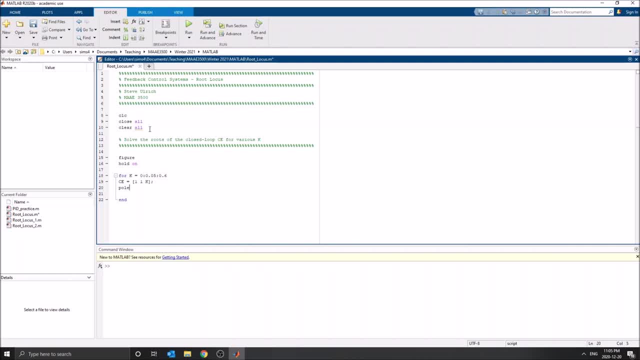 Based on this polynomial. what I'm gonna do now is find the roots, or the poles in that characteristic equation. I'm gonna simply solve for the roots using the MATLAB command roots- Easy peasy. So just to add a bit of comments here: 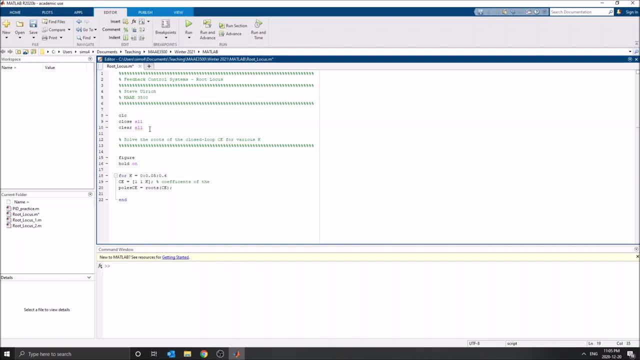 these are the coefficients of the characteristic closed loop characteristic equation in the form of a holding polynomial. All right, And then we're then calculating the closed loop poles, And next I'm gonna plot the poles, first by obtaining the real parts of the poles. 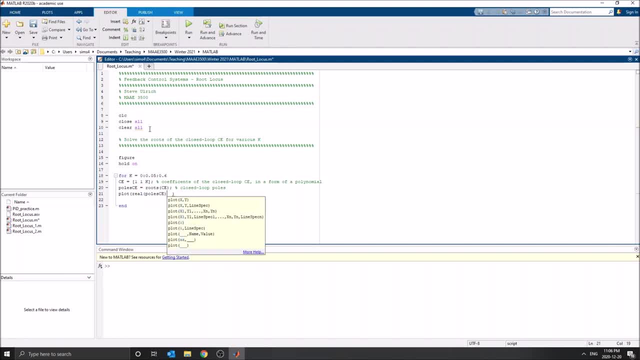 So poles C, E, versus the imaginary components of my poles, or the roots of my characteristic equation, And I'm gonna plot them with little stars. So that's X, And instead of using the default color, which is blue, I like to use black. 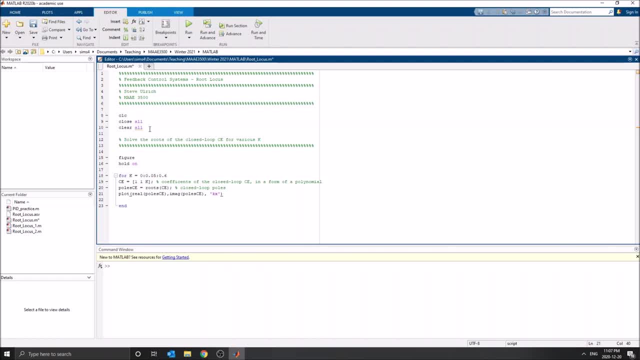 So K for black X to specify that I want the poles to be visualized as stars on the plot. All right, Next I'm gonna set my axis So that I see what's going on. I'm gonna use minus 1.2 to 0.2 along the X-axis. 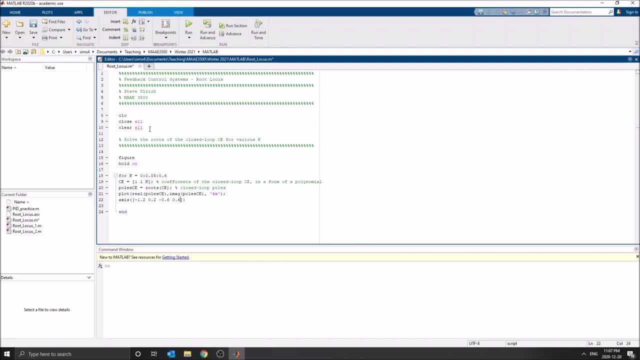 and minus 0.6 to 0.6 along the Y-axis. Now add some grid to better visualize the data. I'm gonna set the label of the X-axis to be the real components of my pole And the Y-label simply be the imaginary component. 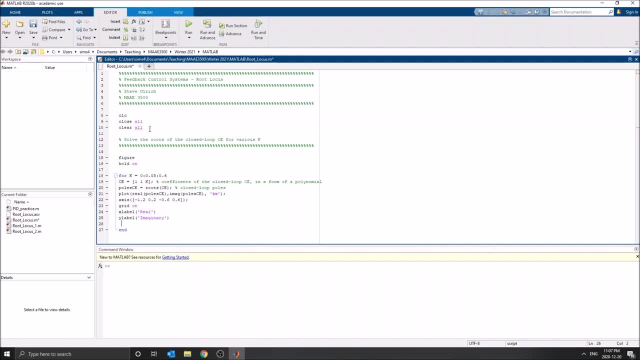 of my poles. Next, I also want to better visualize the location of the open loop poles or the location of the closed loop poles, evaluated at K equal to zero. This is exactly the same thing, So for that I'm gonna simply specify the poles. 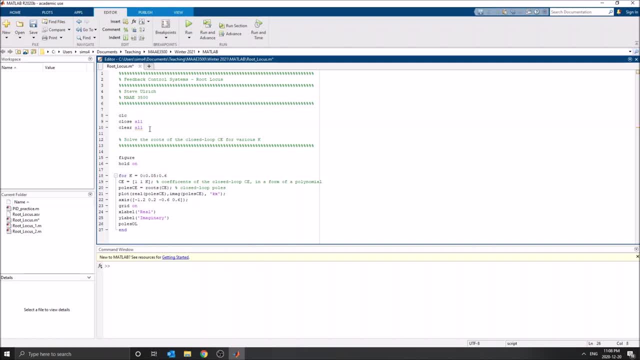 and then I'm gonna plot them. So I'm gonna specify the poles of my open loop system, the open loop as being one. if you remember, we had one at the origin, so zero, and the other one at S, equal minus one. 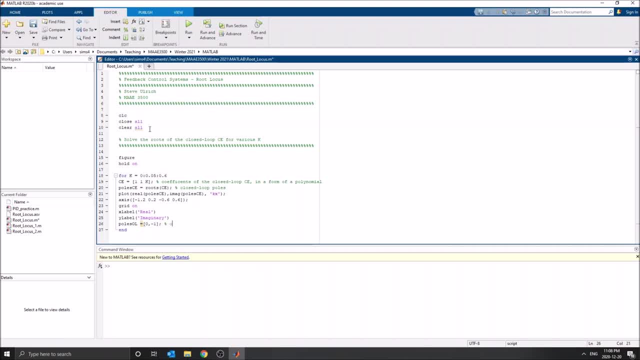 So, just to be explicit, these are the open loop poles, Or in other words closed loop poles evaluated at K equal to zero. So that would be the starting point in the root locus And of course, I want to plot them using the same strategy as we've used before. 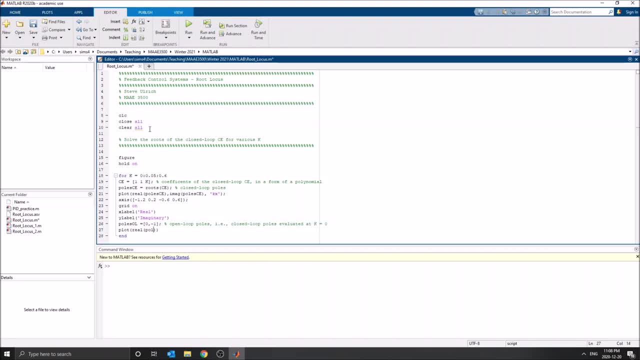 So plotting the real parts of all the poles in the open loop transfer function versus the imaginary part of my poles, open loop This time. to distinguish them from closed loop poles, or whenever K is larger than zero, I'm going to plot them with red stars, like that. 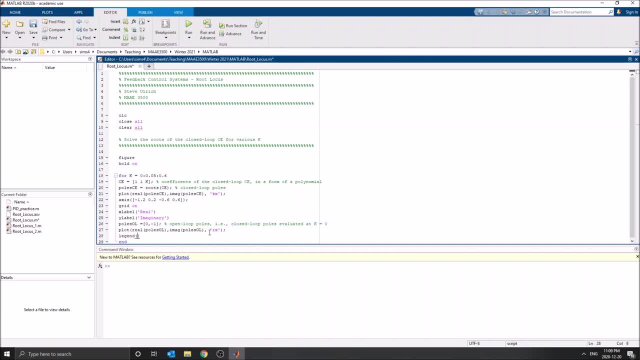 I'm gonna add a legend to better visualize the data, Let's say evaluated for K, equal to the current value of K. within this for loop, I wanna turn this variable, which is num, into a string using the numToString command of this particular variable, K. 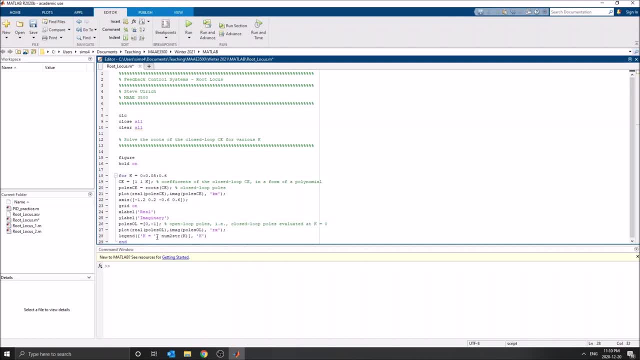 And then I'm also going to specify that for the other piece of data, correspondence to the poles whenever K is equal to zero, and that would be five. that would be for the open new polls, all right, and then give us some time to. 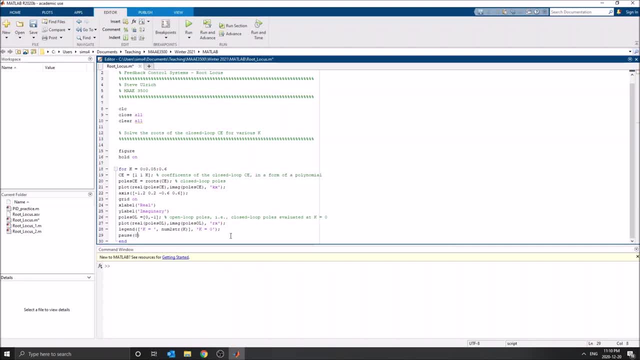 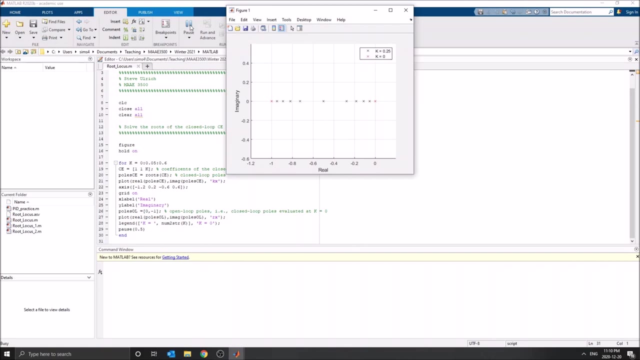 visualize what's going on. I'm gonna pause or say 0.5 seconds between each iteration, and that should be it. so let's see how it looks like. there you go. so you see that as we increase the gain K, the polls moved from their original. 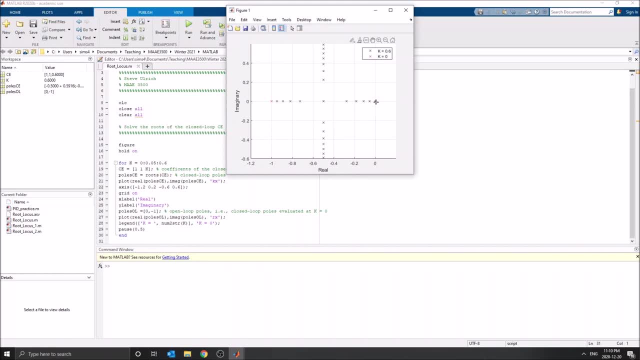 location that corresponds to the open new poll location at s equals 0 at the origin and the other one, at s, equal minus 1, and as K increased from 0 to, in this example, 0.6, we saw both poles smashing into each other, one flying off. 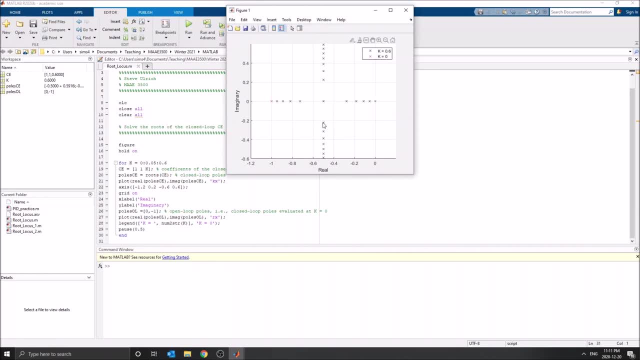 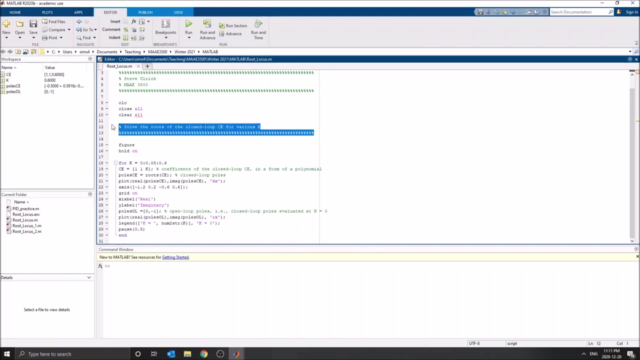 vertically all the way to the top and the other one flying down at the bottom, like that, and that corresponds to what we saw when we solve the root locus manually by following the nine rules. it's just a very efficient way to do it all right, so hope that makes sense. but that's the brute force method, the second strategy. 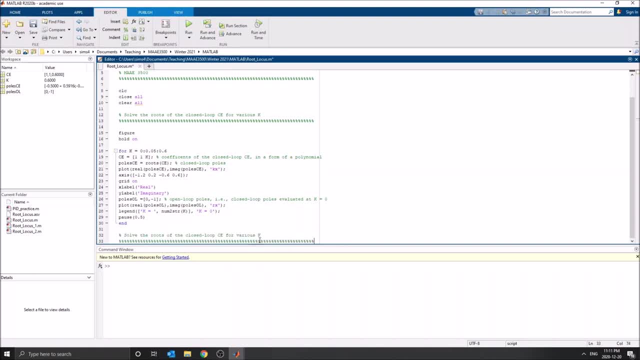 is not to solve for the roots of a characteristic equation manual, as we've just done using a for loop, but instead now we're going to draw the root locus beyond math labs built in command, known as our locust. and if you think that the first strategy was an easy solution, wait. 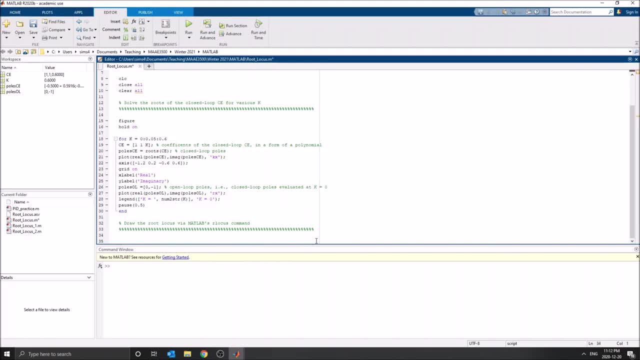 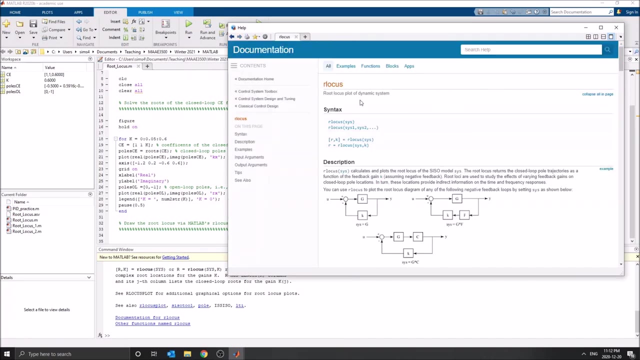 till, you see this one. so math lab, our locust comments. so how does that work? let's find out. help, documentation, let's have a look together. all right, our locus, our locus plot of dynamic system or of transfer functions, same thing. so our locus, cis. so what is cis? cis corresponds to the 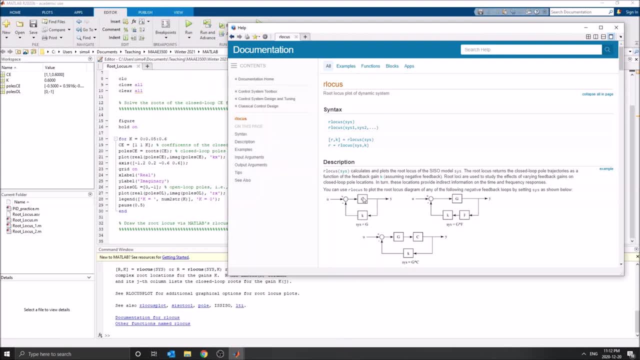 plant transfer function denoted by g in the block scheme diagrams. in our case, this is the plant transfer function that we've denoted as g of p thus far. so all we need is to specify the plant transfer function and automatically what this tells us is that root locus would close the loop. 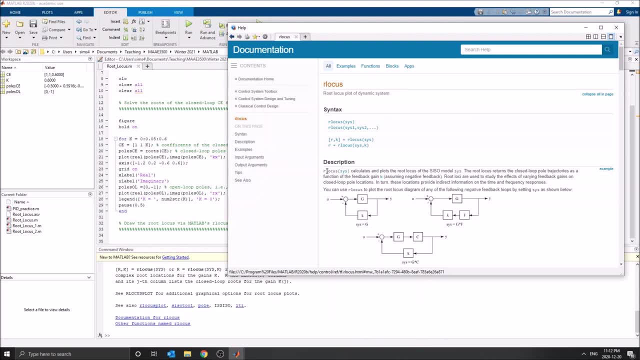 for us. so we don't even need to worry about manually calculating the closed loop transfer function, finding the characteristic equation and things like that. all we need to specify is the plant transfer function. so that is beautiful. okay, our locus of cis calculates plot and plots the root locus of the cso, which stands for single input. 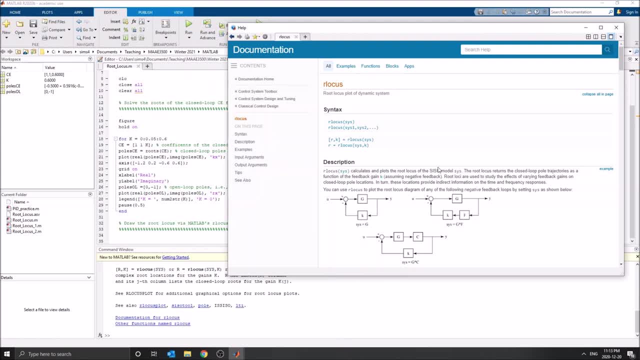 single output, model six. that's just what i've described. uh, take note that single input, single output only means that this is a system that can be modeled using transfer functions, and that's what we've been doing so far. this is uh in opposition to mimo systems, which would stand 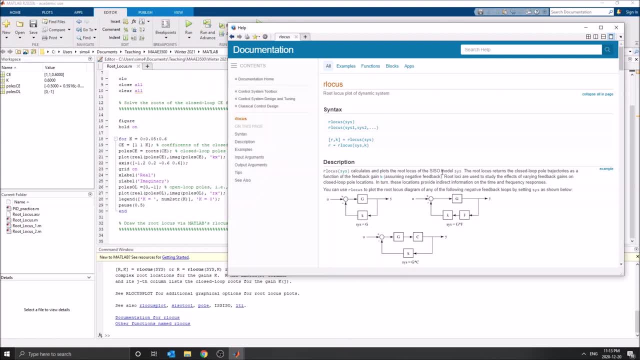 for multiple inputs. multiple outputs where you would need to use state space representations to model such systems, but that's beyond the scope of this. uh, this lecture. okay, but wait, look at these architectures that matlab, our locus command, assumes. none of them corresponds to what we've assumed so far, where the static gain k. 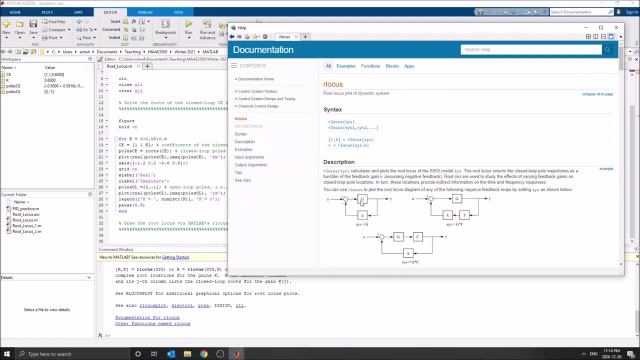 with the plant transfer function g of p. so instead, matlab r locus function assumes that this gain is in a parallel configuration with the plant. oh, is that a problem? well, let's go back to the whiteboard and analyze that further. all right, so let's find out together. 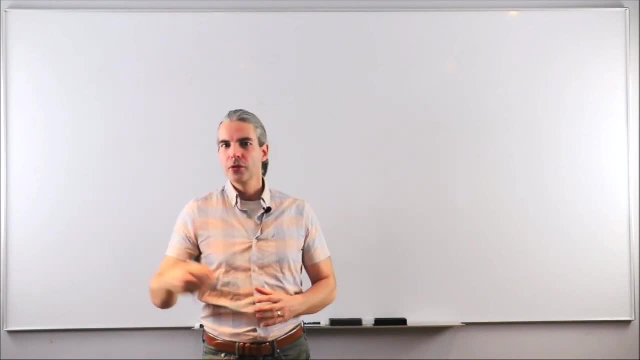 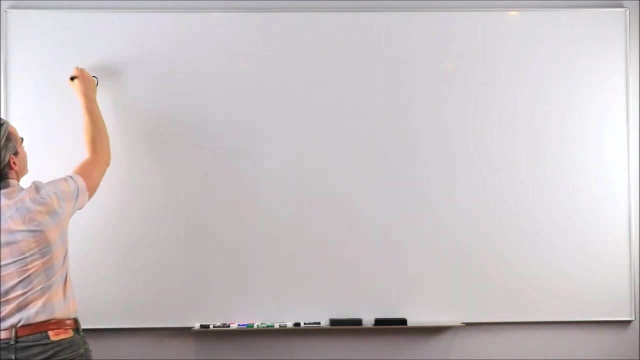 if, using the math that built-in function r locus would create some issues or problems because, as we've just seen, together the architecture that our approach assumed in the past, in what matlab assumes as the underlying architecture behind the root locus matlab function, then there's a discrepancy. so let's have a look at that. our architecture, as always, is the reference signal. 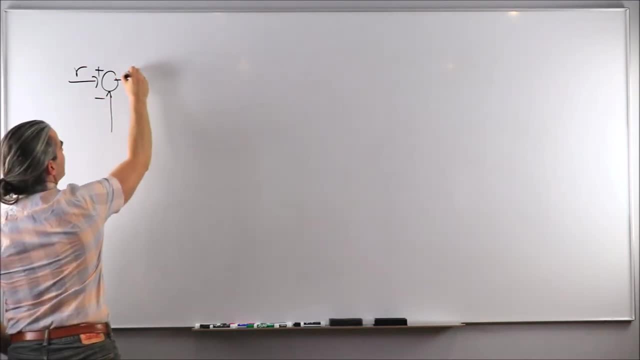 being compared to the plant output. that creates an error. an error is being multiplied by some proportional control action that creates a control denied by us control. does that? three sub code are more than enough to create a? to take 6 different signal nodes that are used in a 24-percent control. 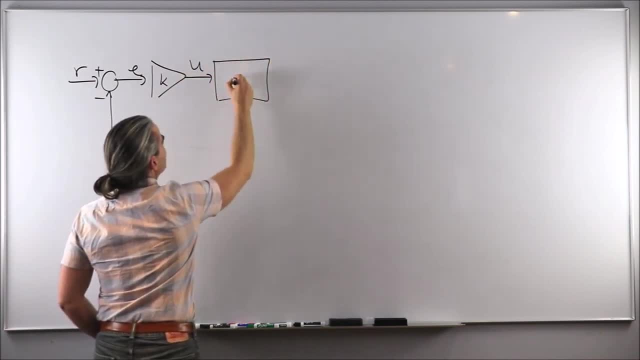 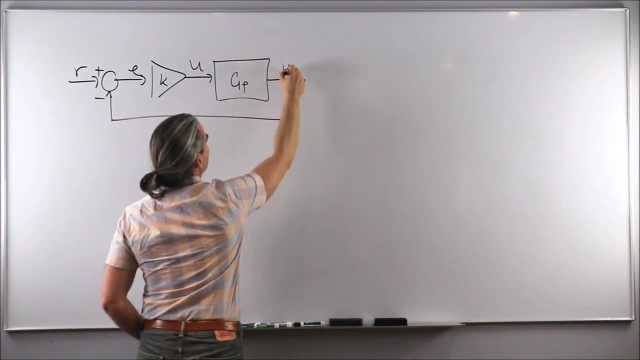 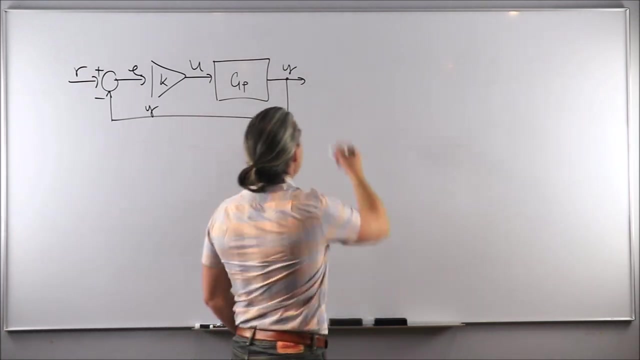 as we've just seen together the architecture that our approach assume in the past. in a control input signal this is being fed for a plant transfer function g of p. that creates a new output signal denoted by y and y over here. on the other hand, MATLAB assumes the following: 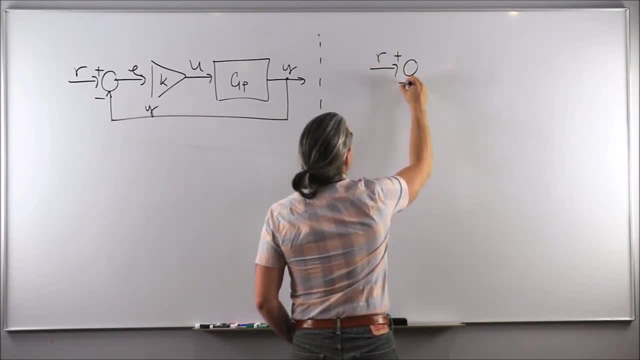 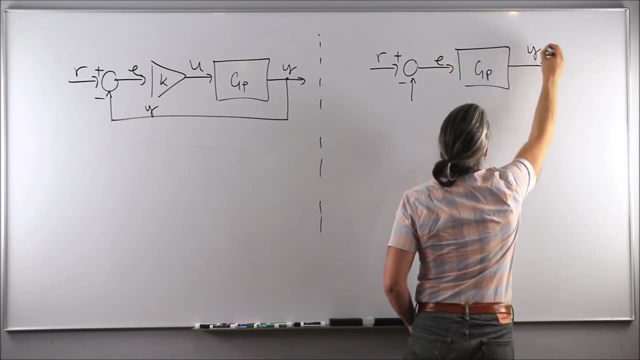 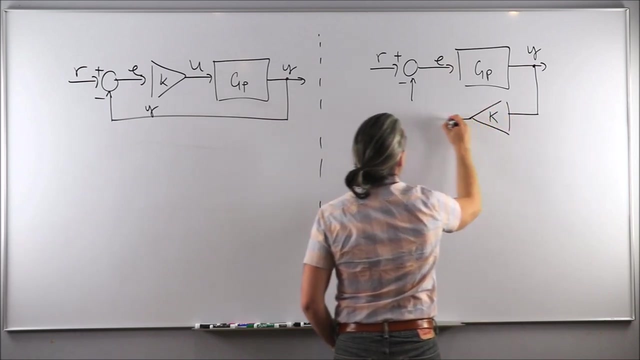 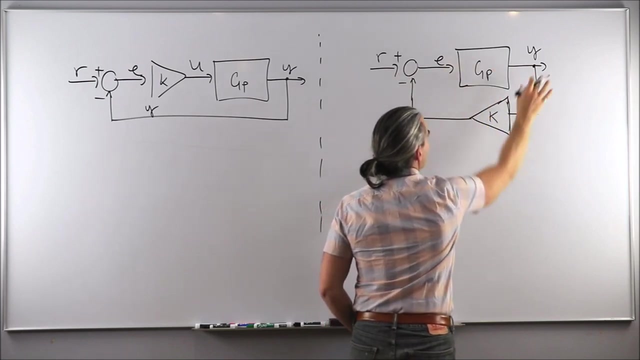 you have the reference signal, plus, minus, you have the error. but then the error is being fed directly into the plant transfer function to create a new output. this output is being multiplied with the proportional control action k, yet not in in the open loop, uh, or the direct path as we've assumed here. it is not in series, but rather in parallel. 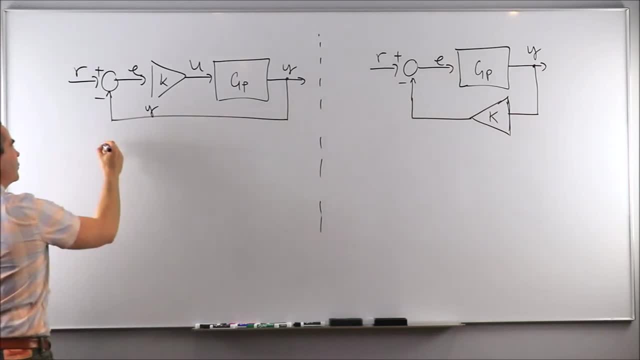 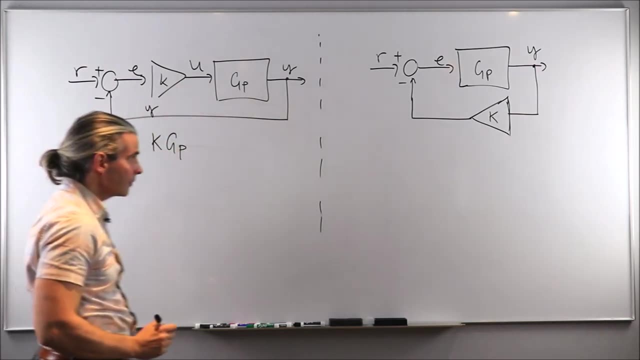 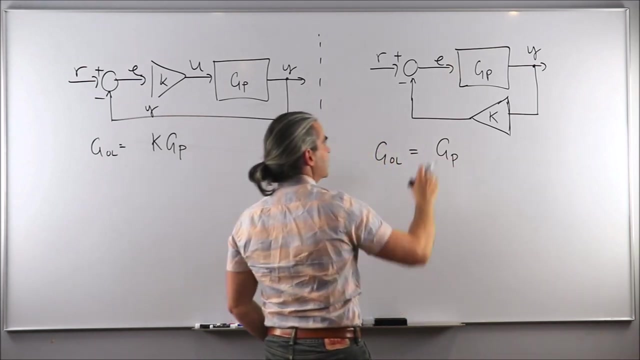 so is that an issue? well, let's find out here. if you look at the open transfer function, we have k times g of p, but, as i've just mentioned, on this side the open loop is simply g of p, because the control action is not in series with the plant transfer function. 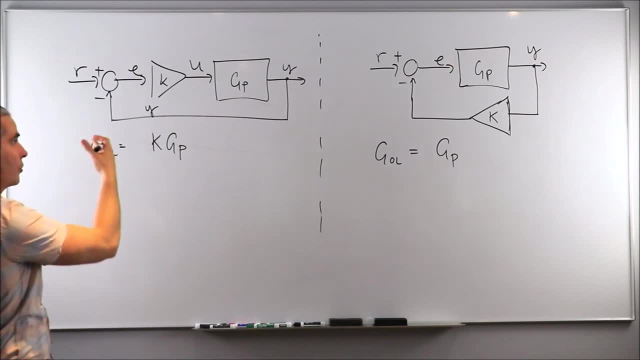 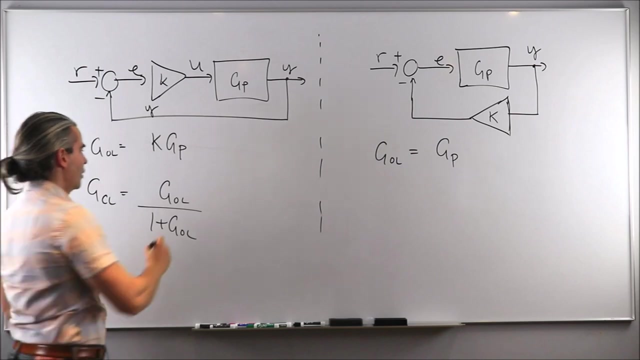 so right away we know that there is a big difference between both architectures. now, if we compare or calculate the closing transfer function, whenever we have this kind of series arrangement, transfer functions, we multiply together. we know by now that this is simply g open loop over one plus g open, or in other words, 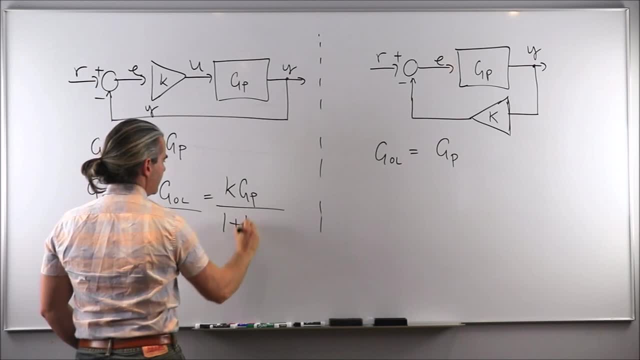 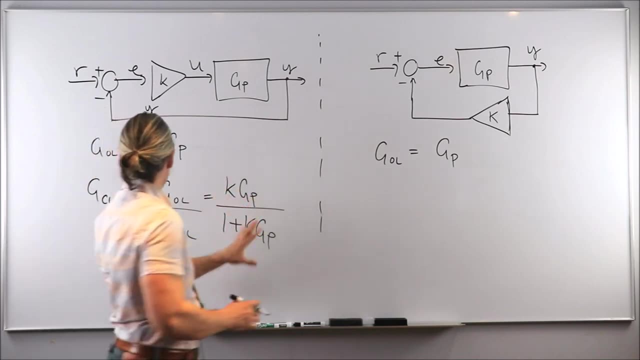 k times g of p, over one plus k times g of p. we've done that literally millions of times. okay, on this side, though, the best way to do it, if you're not sure, is just to essentially simply chemically cell eclipse the decay of mu and then cuff Lankel or link hydrogen minimum if you know how to nervous to gross 어렵ulation, or if you're just learning outputگ available to you, for example, 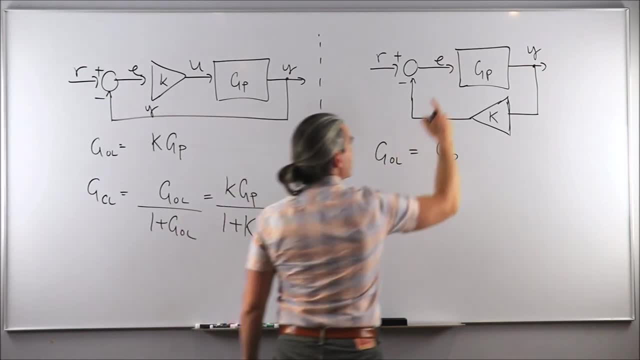 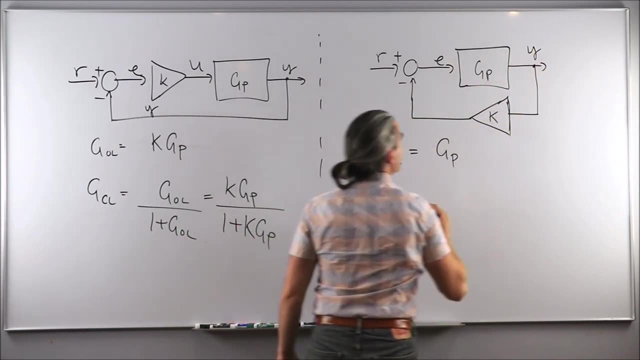 the best way to do it if you're not sure, is just to demonstrate how you can- zu- literally can- omit g, ultimately inained g- to write out what all the signals would be equal to, and I like to start the process always with the output signal y. 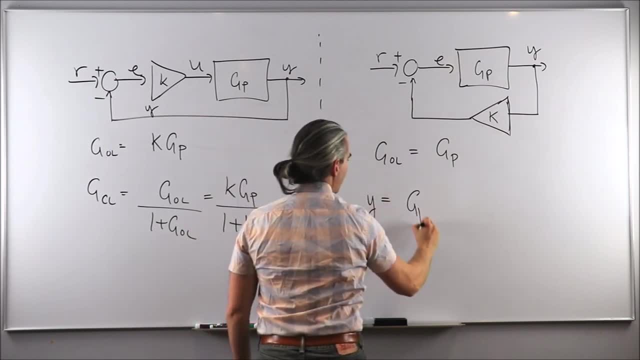 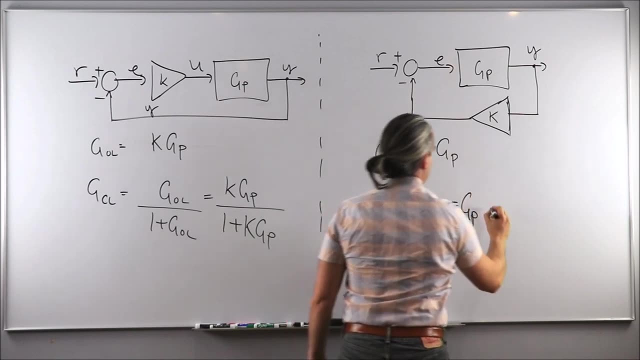 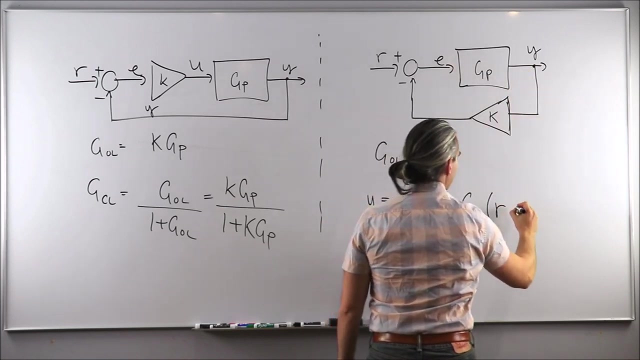 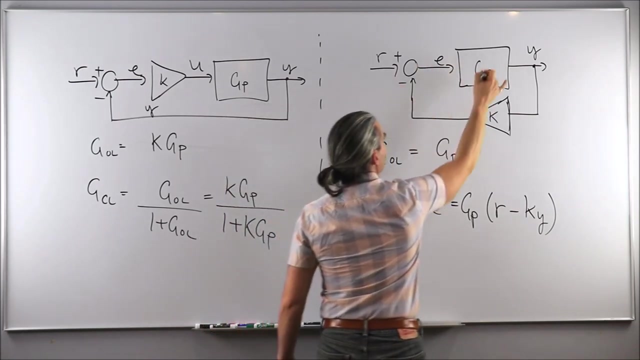 So I'm gonna write that y is equal to gp times the error. But we know that the error is calculated as r minus y times k or minus k times y. And now I went through all the paths or I've closed the loop. 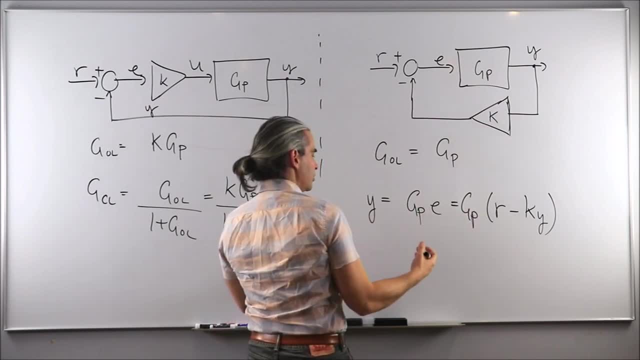 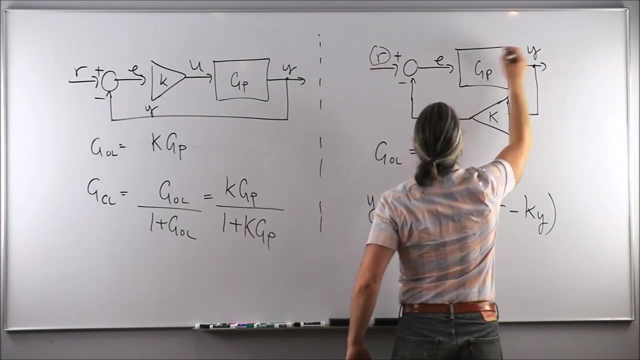 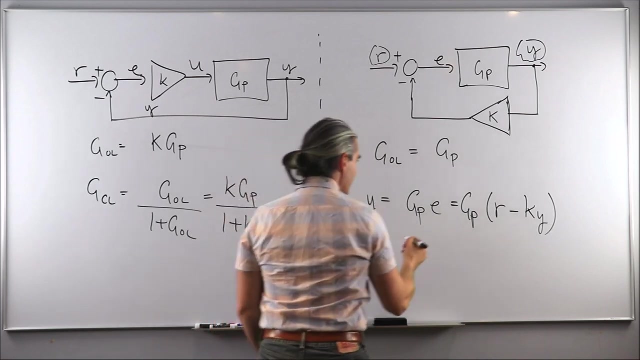 by writing this equation essentially, and now I'm in a good position to solve for the mapping between, again, the global output r, the global input r to the global output y, or in other words, finding the closing transfer function manually. 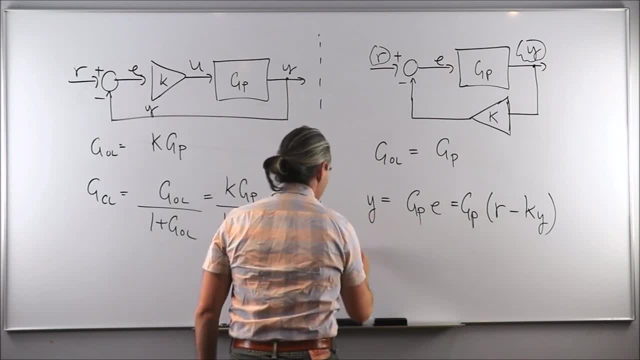 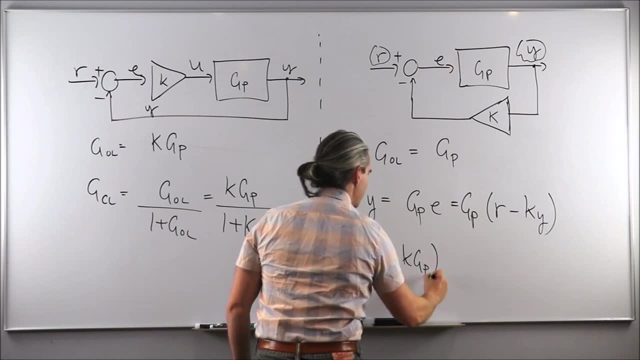 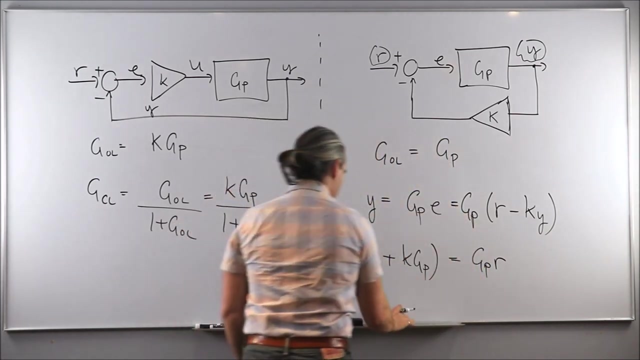 I'm gonna put all the y terms on one side. I'm gonna solve for it. so y one plus k, k times g of p, being equal to g of p times r, If you want the closing transfer function. this is nothing more. 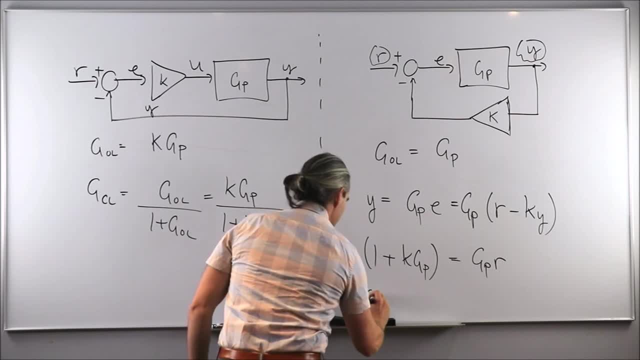 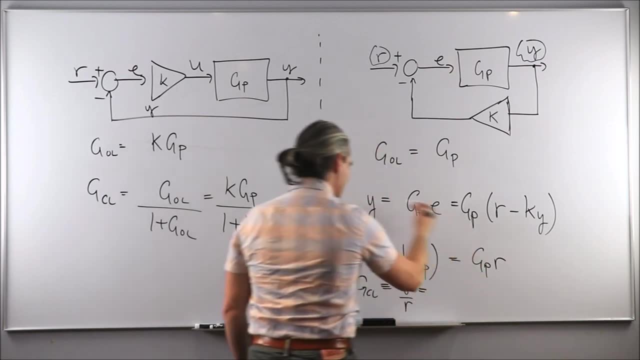 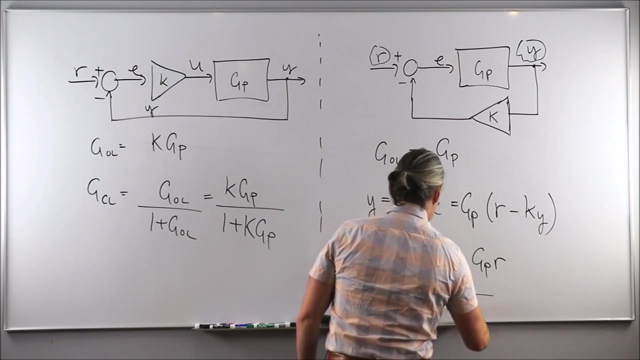 So g closed loop is being equivalent to y over r and that, based on that equation, is simply given by g of p times r times one plus k. g of p Closing transfer function for the MATLAB architecture behind our locus function. 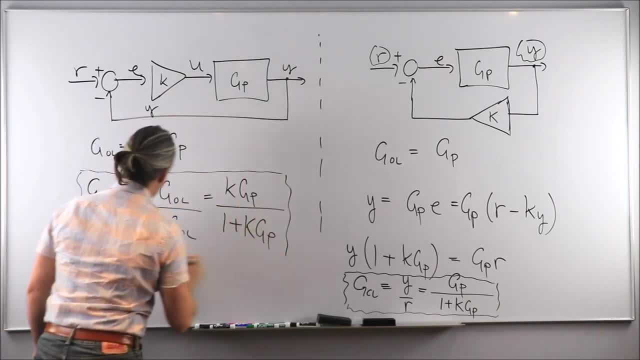 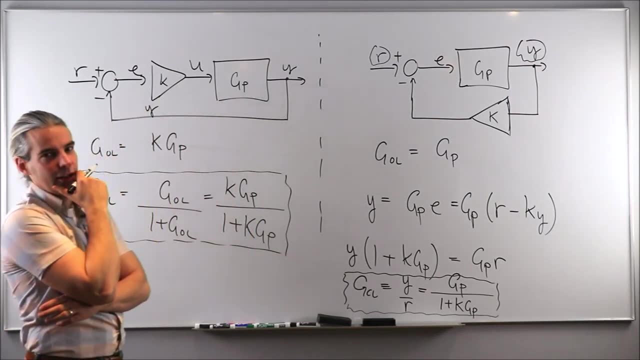 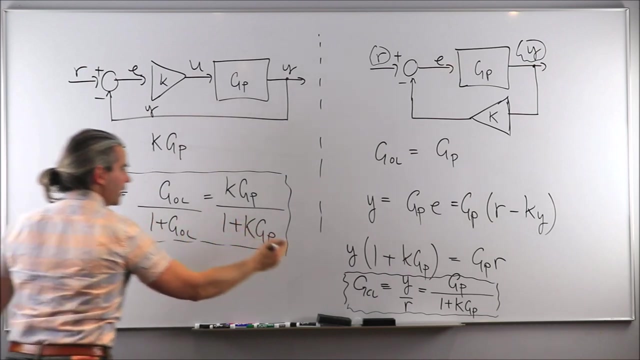 compare that to our closing transfer function, obtained based on our architecture that we've used throughout this course. Gee, it's not looking good. Well, it's not that bad because you know, if you compare what matters- and what matters is not the transfer function- 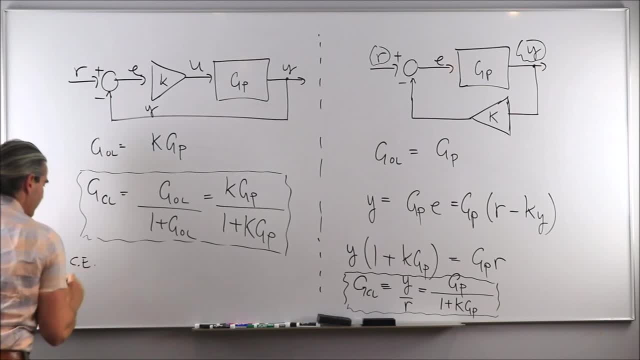 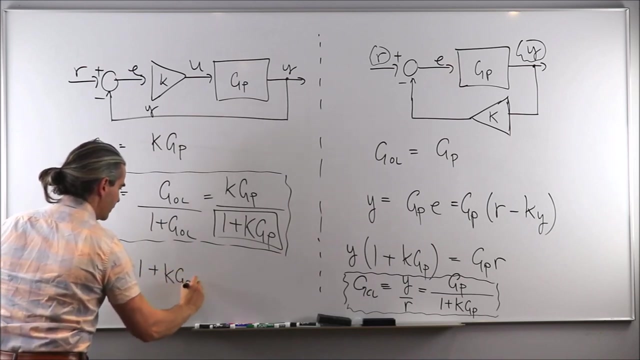 but the characteristic equation, Characteristic equation of g- closed loop, is going to be equal to the denominator of the closing transfer function. So one plus k, g of p, always equal to zero. And if you look at what we have here, characteristic equation of g- closed loop, 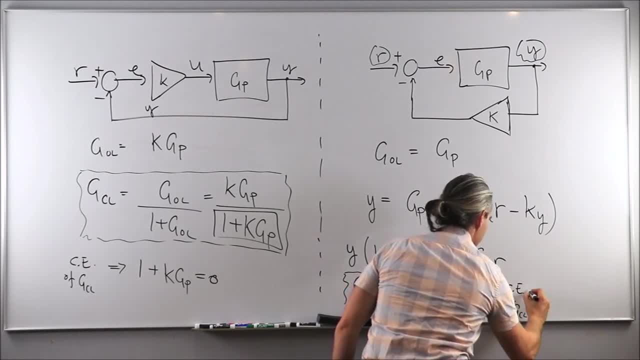 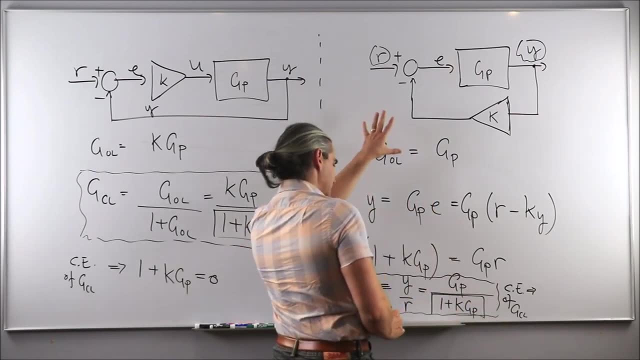 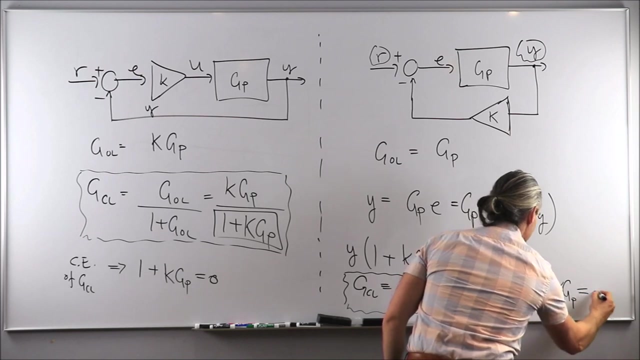 is going to be the denominator of our closed loop transfer function for this specific architecture. So one plus k, g of p equal to zero, And this is like magic, right? So if you look at what we have here, we have a characteristic equation of g- closed loop. 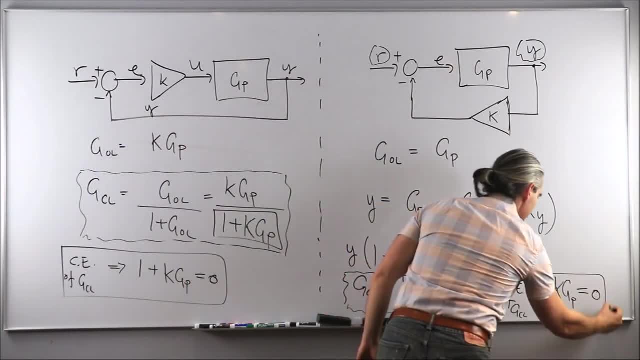 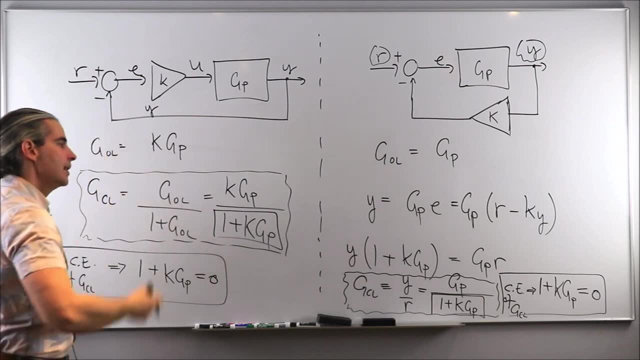 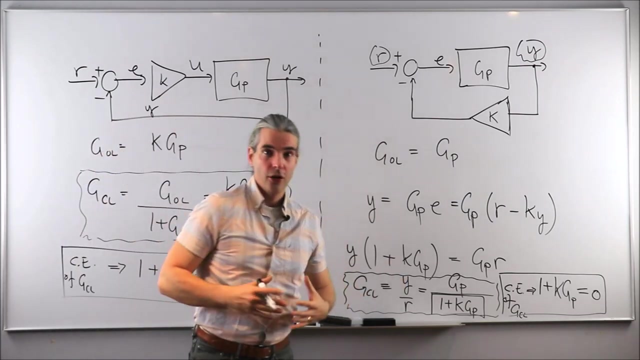 which is equal to zero Right. Because although the opening transfer functions were different, compared this to that they're not the same. And although the closed loop transfer functions were also different, turns out that the denominator of both closed loop transfer functions are exactly the same. 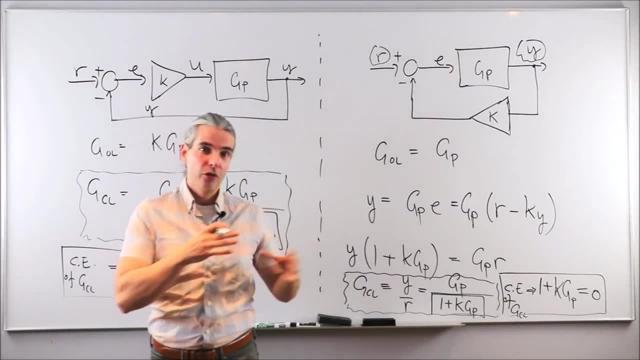 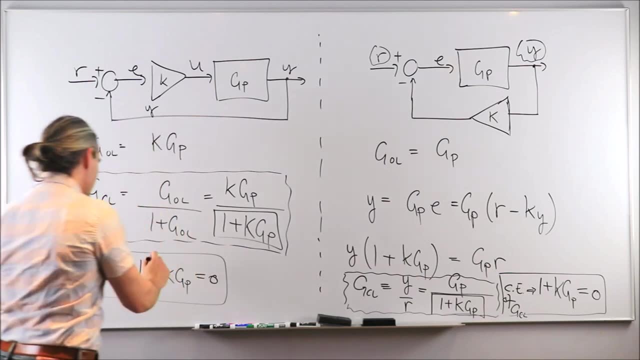 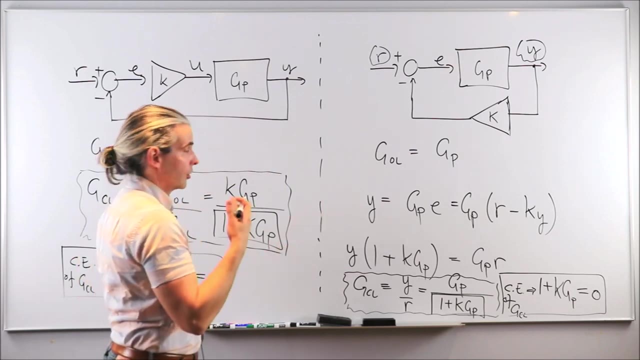 Or in other words, the characteristic equation of both architectures is exactly the same. It's one plus k g of p, one plus k g of p- zero, And that means that the roots of those characteristic equations are going to be exactly the same. 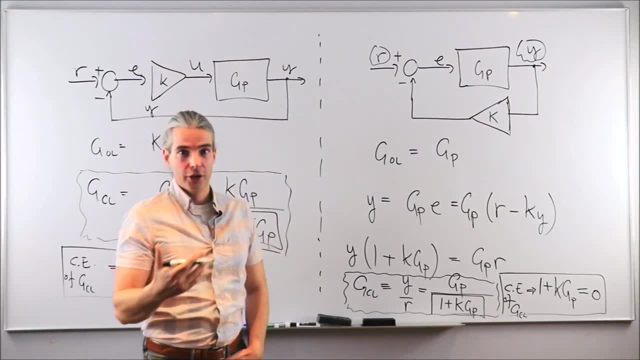 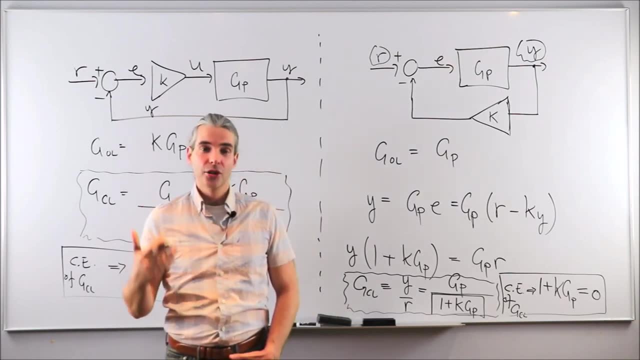 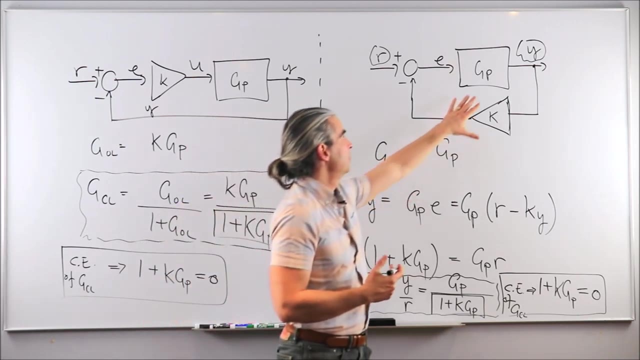 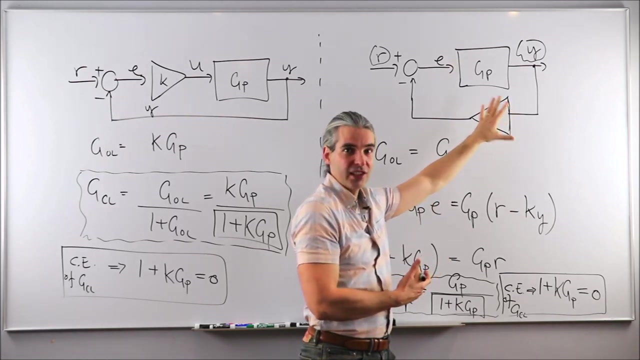 Or in other words, the poles of the closed loop transfer functions will be exactly the same in both situations. So the answer is yes. We can confidently use MATLAB RLOCUS function, even though the built-in architecture that MATLAB assumes whenever we type RLOCUS- 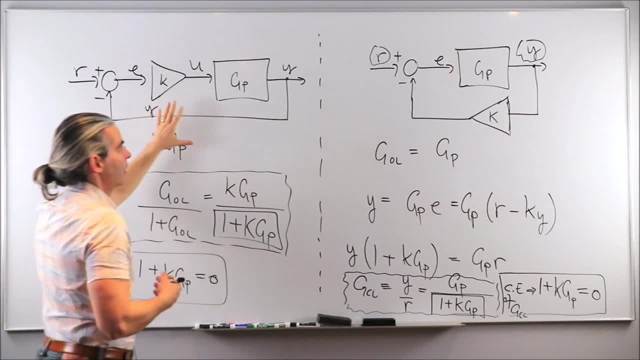 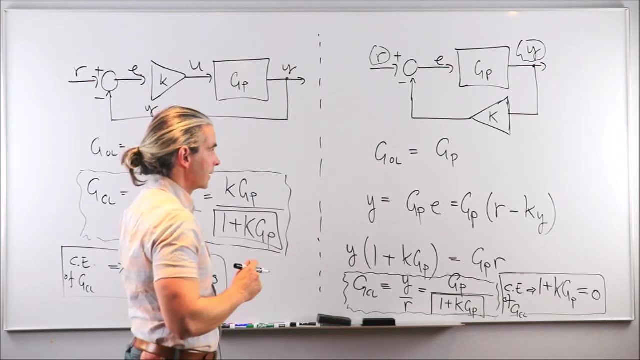 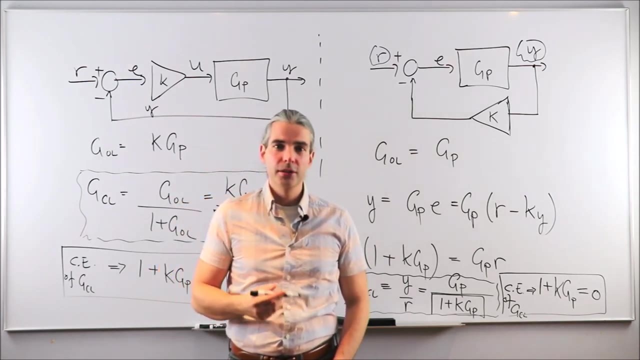 is different than what we had used so far in terms of constructing the ROOTLOCUS manually by going through the nine rules. All right, good news. So let's go back to the computer and let's let MATLAB do the ROOTLOCUS for us. 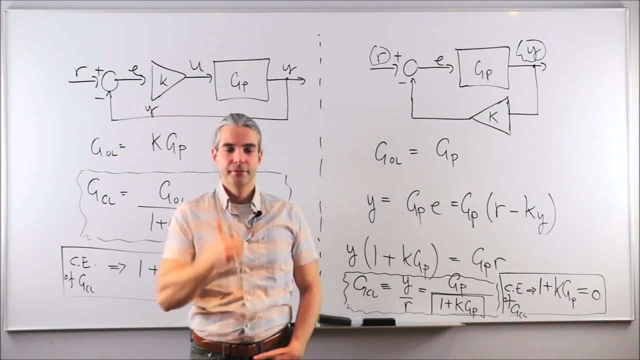 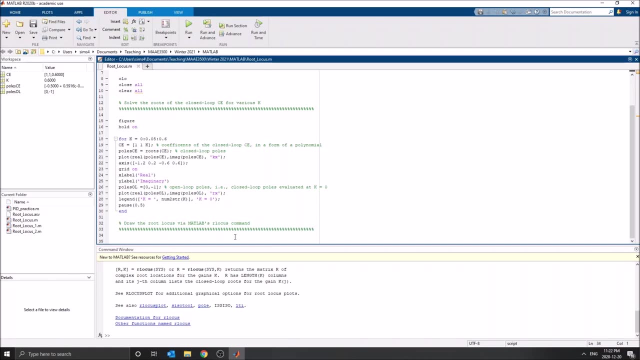 by using the RLOCUS command. Let's do that together. Okay, So in MATLAB, as we've seen on the whiteboard, using the RLOCUS command is not an issue at all, although the architectures are different. So let's use the RLOCUS command. 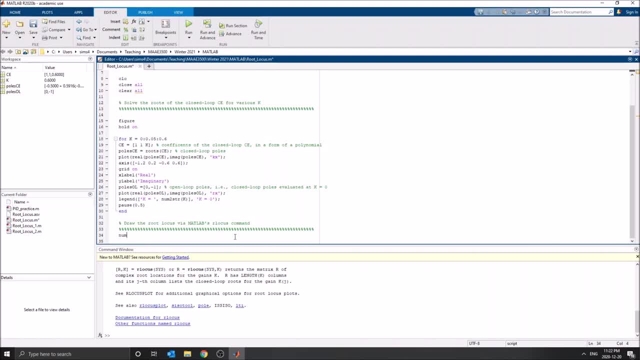 to draw the ROOTLOCUS for us. Let's see how easy it is. So, as we've discussed, all we need to specify is the plant transfer function g of p, And the way we do that, as you know, in MATLAB, is by specifying the numerator as a polynomial. 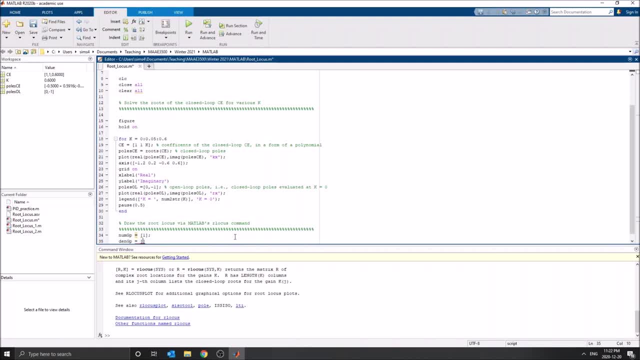 Okay, And then specifying the denominator as another polynomial, And in our case our plant transfer function was simply one over s times s plus one, Or, in terms of polynomials for the denominator, this is s squared plus s plus zero. Okay. 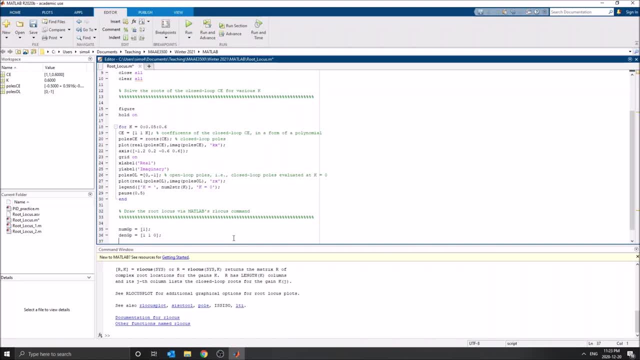 Now that we've defined the numerator and denominator of our transfer function for the plant, we need to create the proper transfer function out of these two pieces, And we do that by using the MATLAB built-in command known as tf for transfer function. 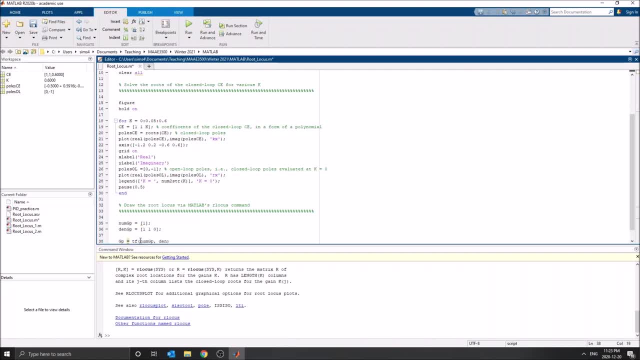 by using the numerator and the denominator of that transfer function, And then all we have left to do is to use the- we're going to create another figure- and to use the RLOCUS command based on our plant transfer function that we've denoted as g of p. 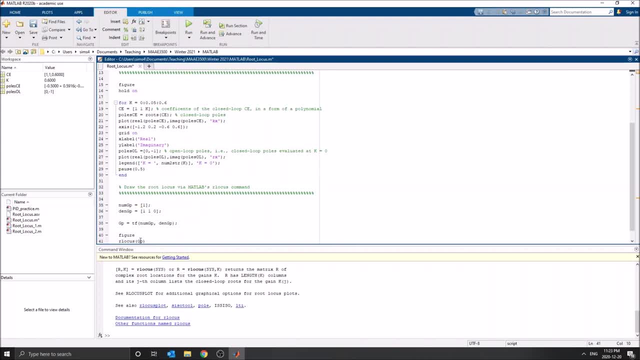 If you go back to the MATLAB RLOCUS documentation, this is referred to as the sys variable. Okay, So again, what it does is that backdoor MATLAB would close the loop for us and apply a static gain k to our transfer function. 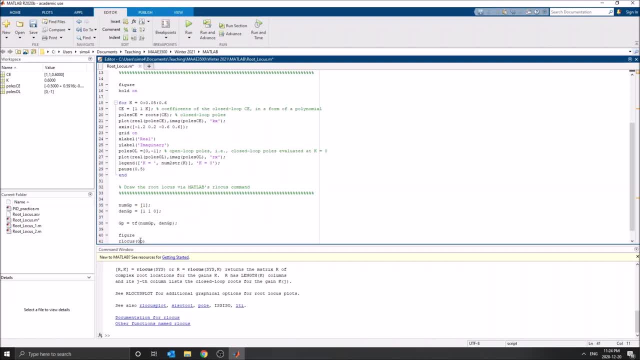 and let k increase from zero all the way to infinity and plot the poles of the resulting characteristic equation, or the roots of the resulting characteristic equation, at each iteration of the gain. So, essentially, RLOCUS does this job for us. 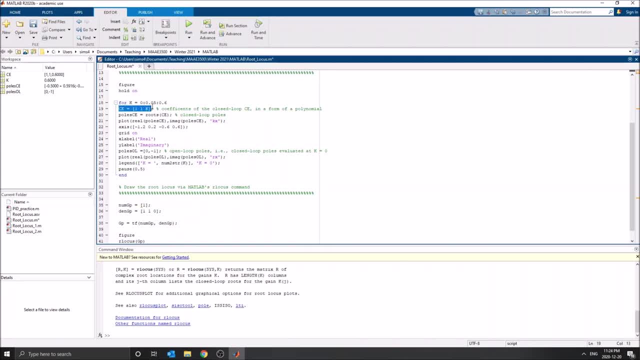 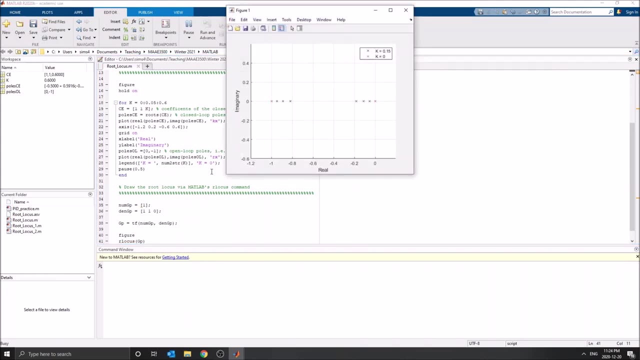 So we don't even need to worry about specifying the characteristic equation, extracting the roots, plotting them, and so on, and so on. A single command, RLOCUS, does it all for us. So let's see how it works. So this is the root force approach again. 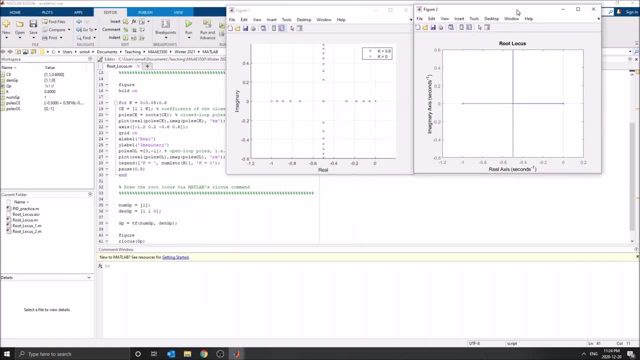 versus the RLOCUS command And, as you can see, both approaches give the exact same results. obviously, All right. It's just a neat way to quickly obtain a root locus for any plant transfer function that you can think of. What's next? 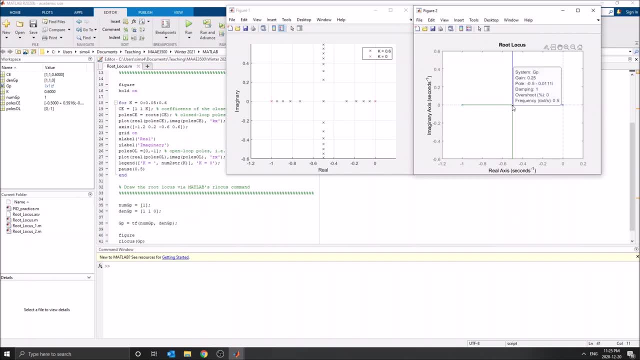 What's neat about it is that you can click on any point on the root locus and you're gonna get several details related to that point. For example, here I've just clicked at the intersection: Gives me the pole locations exactly. Gives me the gain for the static gain k. 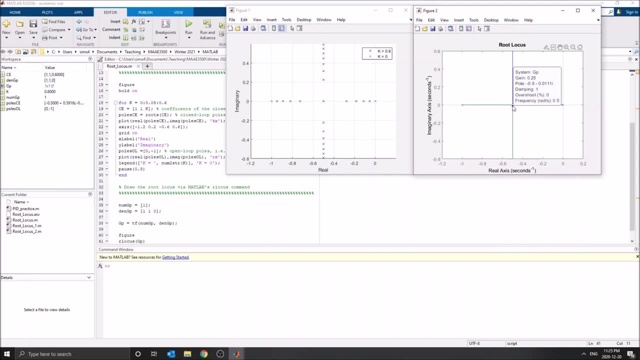 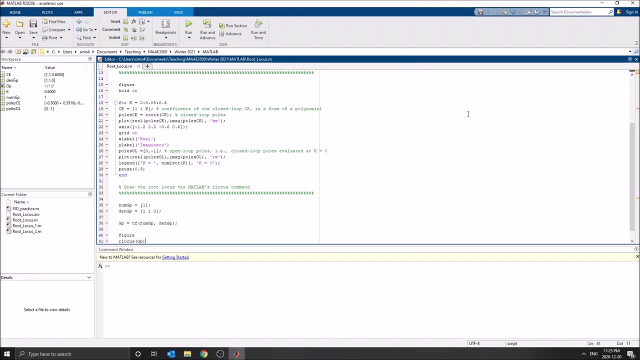 that drives the pole at that location, An application that gives me the damping ratio, zeta, The overshoot in terms of percent And the natural frequency, 0.5.. All right, So now that we've learned how to use the MATLAB. 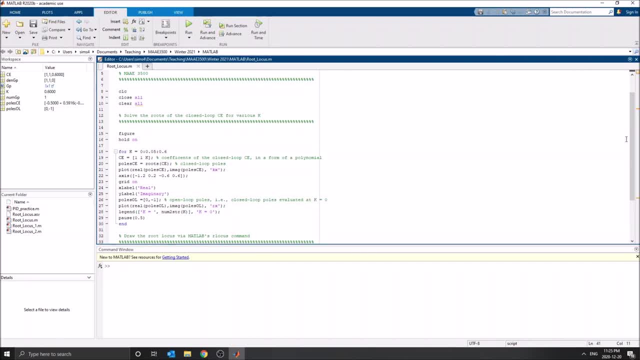 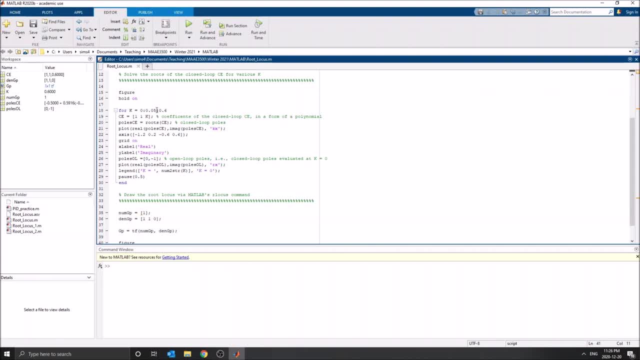 And again we'll compare both methods or approaches: the root force method and using the command. So first I'm gonna change a little bit my increment for my gain value that I wanna look at. I'm gonna go from zero this time all the way to 10. 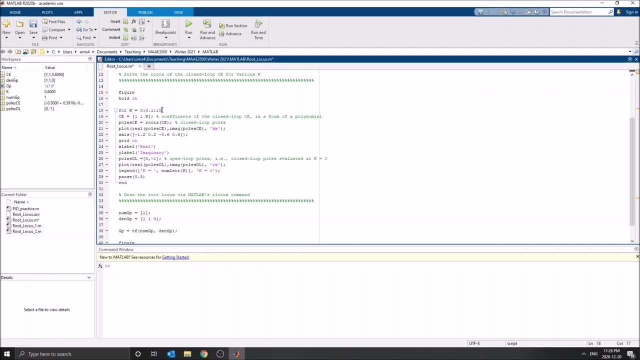 so that we can see some interesting behavior of the root locus. We'd have to go all the way to 10 in that case. The characteristic equation for the second example, if you go back to that lecture, it was s cube plus three s. 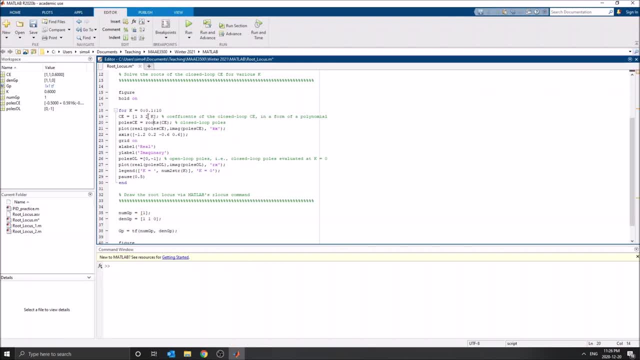 square plus 2s plus k. all right. now i'm going to change my axes a little bit in terms of their limits so that we can clearly see the full root locus. i'm going to go minus 2.5 to 0.2 and say: 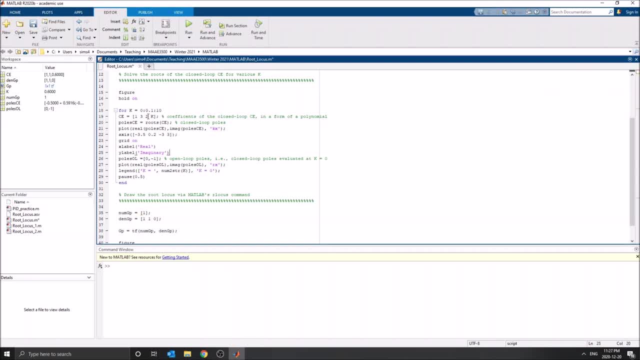 minus 3 to positive 3. again, my labels don't change. the open new poles in that case were 0, s equal minus 1 and s equal minus 2.. all right, and because i have so many points- in that case i have 100 points- essentially i'm gonna plot, i'm gonna pause for a shorter period of time.